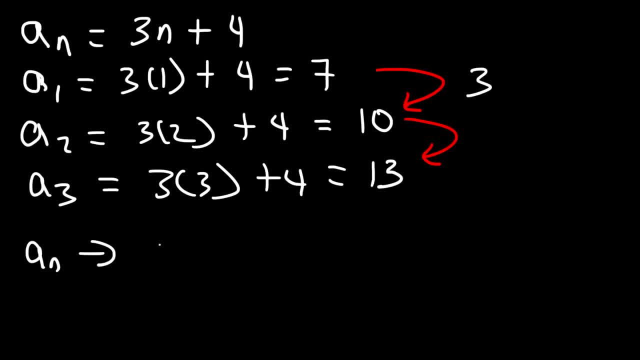 So if we list out the terms of the sequence, we see the first term is 7,, the next term is 10,, the third is 13,, the fourth is going to be 16. And so forth. So, as n approaches infinity, what happens to the value of the sequence? 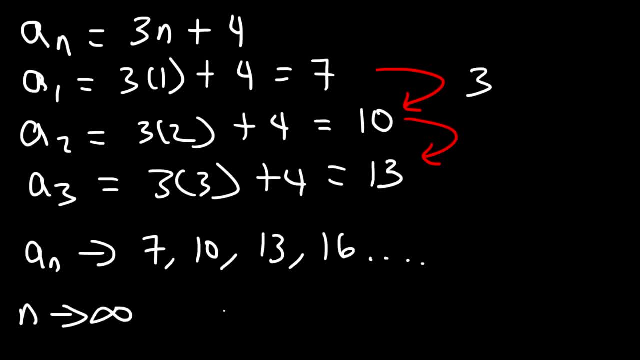 Notice that it's increasing without bound, So the value of the sequence will go all the way up to infinity. It's going to keep getting higher and higher And, as a result, we say that the sequence diverges because it doesn't converge into a specific number. 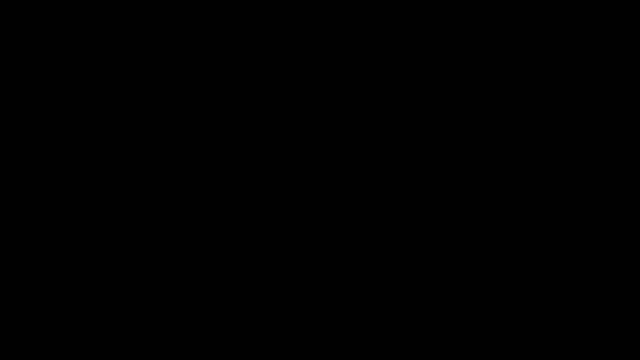 It keeps just getting higher and higher, And so you need to understand this: The limit as n approaches infinity for a sequence. if it approaches a specific number- let's call it L- then we say that the sequence converges. There's a difference between a series and a sequence, but the sequence converges. 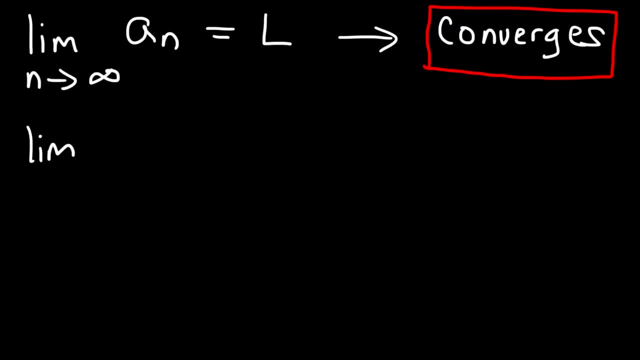 Now let's say: if, as n approaches infinity for a sequence, it doesn't exist. Or let's say it increases without bound or decreases without bound. In that case the sequence diverges because it doesn't converge to a specific number. 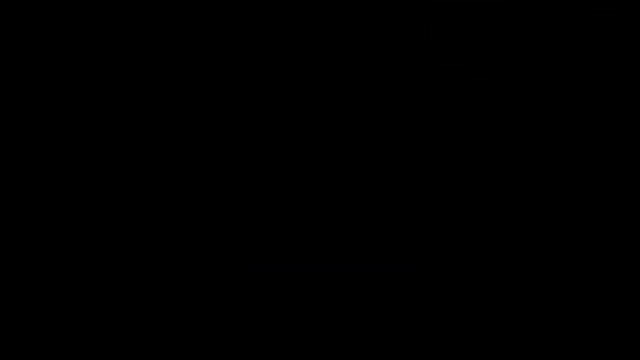 Now let's look at another example. So let's say, if we have the sequence a sub n is 1 over 3 to the n. So does the sequence converge or diverge? What would you say? Well, let's write out the first four terms. 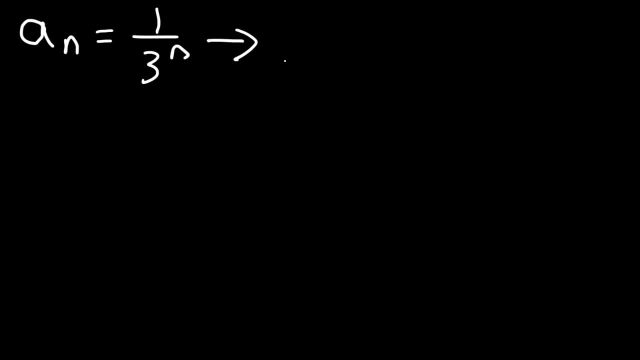 So a sub 1, that's going to be 1 over 3 to the first power, or simply 1 over 3.. And then the second term, a sub 2,, that's 1 over 3 squared, and 3 squared is 9.. 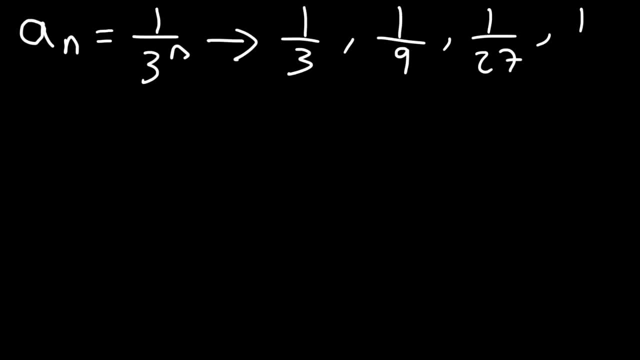 The third term, 3 to the third, is 27, and the fourth is going to be 1 over 81.. Now let's get the decimal values for these numbers, Okay, So 1 over 3 is basically 0.3 repeating. 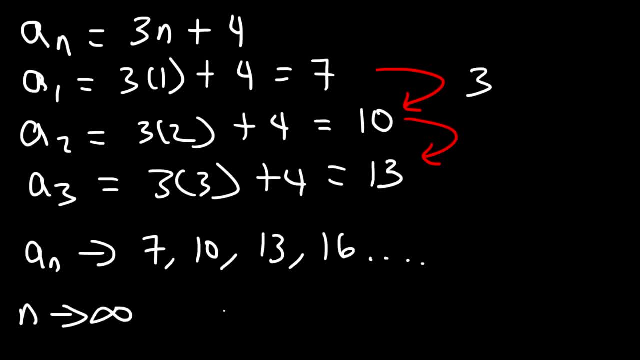 Notice that it's increasing without bound, So the value of the sequence will go all the way up to infinity. It's going to keep getting higher and higher And, as a result, we say that the sequence diverges because it doesn't converge into a specific number. 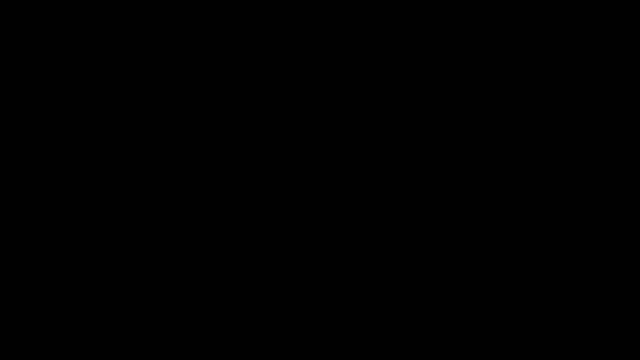 It keeps just getting higher and higher, And so you need to understand this: The limit as n approaches infinity for a sequence. if it approaches a specific number- let's call it L- then we say that the sequence converges. There's a difference between a series and a sequence, but the sequence converges. 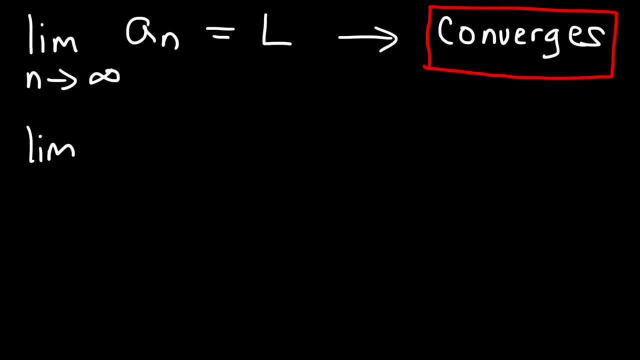 Now let's say: if, as n approaches infinity for a sequence, it doesn't exist. Or let's say it increases without bound or decreases without bound. In that case the sequence diverges because it doesn't converge to a specific number. 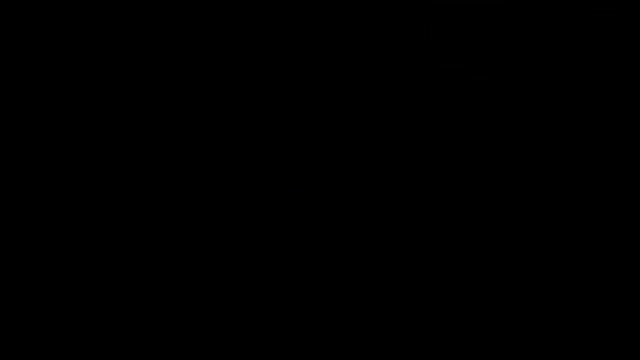 Now let's look at another example. So let's say, if we have the sequence a sub n is 1 over 3 to the n. So does the sequence converge or diverge? What would you say? Well, let's write out the first four terms. 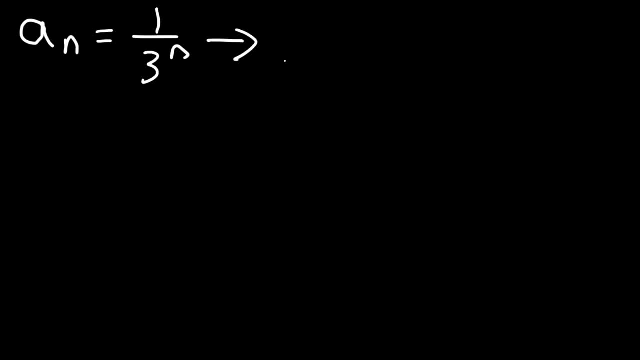 So a sub 1, that's going to be 1 over 3 to the first power, or simply 1 over 3.. And then the second term, a sub 2,, that's 1 over 3 squared, and 3 squared is 9.. 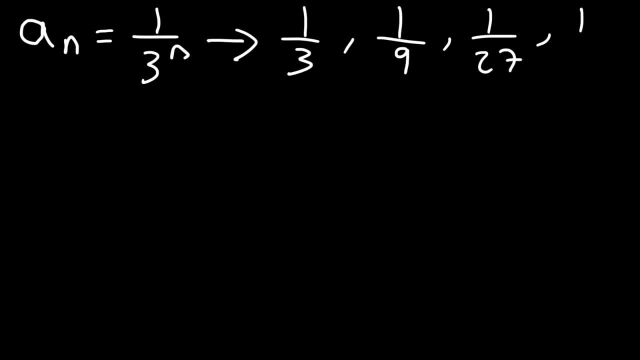 The third term, 3 to the third, is 27, and the fourth is going to be 1 over 81.. Now let's get the decimal values for these numbers, Okay, So 1 over 3 is basically 0.3 repeating. 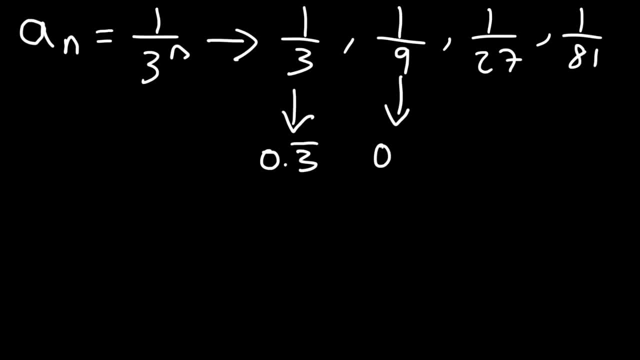 And 1 over 9, that's 0.1 repeating, And the next one that's going to be 0.037 repeating, And then 1 over 81, it's like 0.0123456.. So I'm going to stop it there. 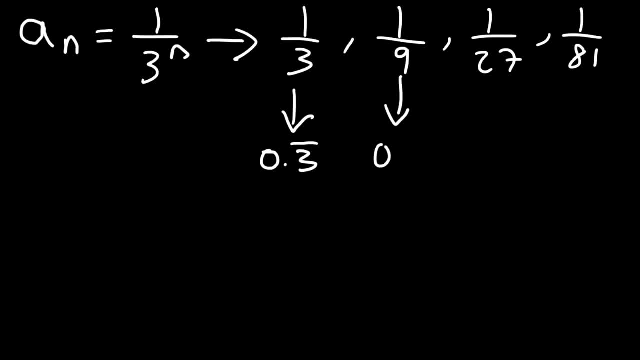 And 1 over 9, that's 0.1 repeating, And the next one that's going to be 0.037 repeating, And then 1 over 81, it's like 0.0123456.. So I'm going to stop it there. 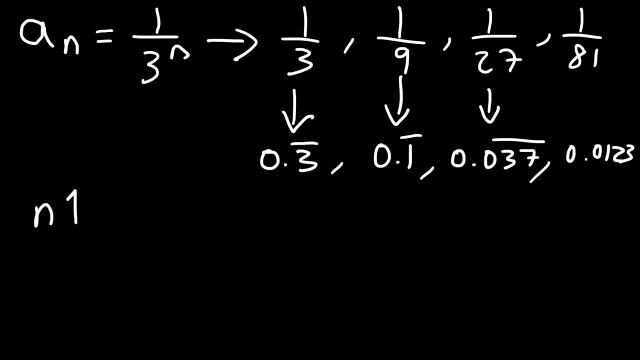 Okay. So notice that as n increases, a sub n is decreasing. In fact, as n approaches infinity, a sub n approaches 0.. So because it's approaching a specific number, we could say that the sequence converges. So we could say that the limit as n approaches infinity, for 1 over 3 to the n, is 0.3.. 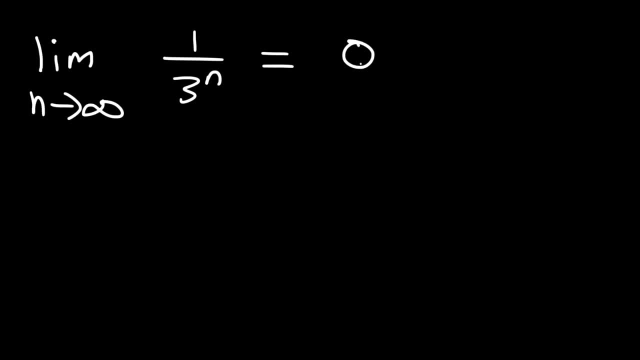 Okay, All right. So now we have a sub n converges to 0.. So the sequence converges And that's the answer. Now let's try another example. So let's say that we have a sub n is equal to 8n divided by 3n minus 5.. 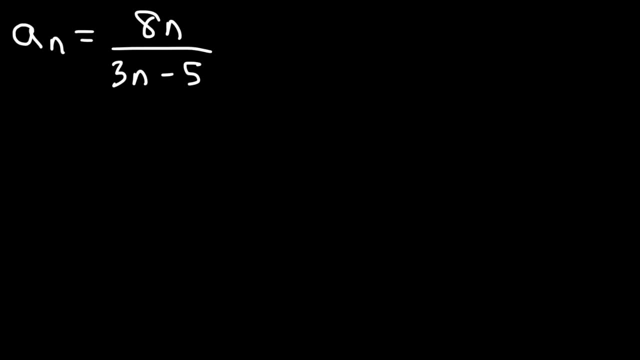 So feel free to pause the video and determine if this sequence converges or if it diverges. So we need to find the limit as n approaches infinity. Okay, So we're going to find the limit as n approaches infinity for this sequence. So what type of algebraic steps can we do here? 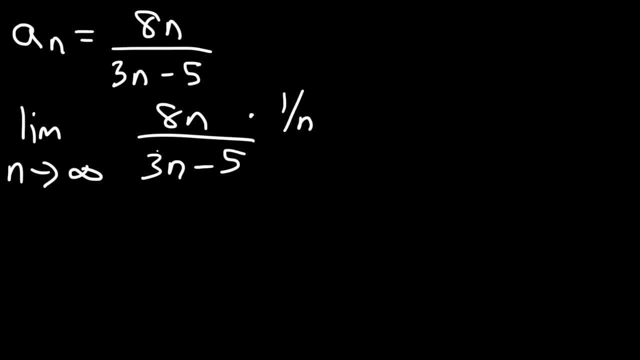 What we need to do is multiply the top and the bottom by 1 over n, And so we're going to get 8 divided by 3 minus 5 over n. Now it's important to understand that the limit as n approaches infinity of something. 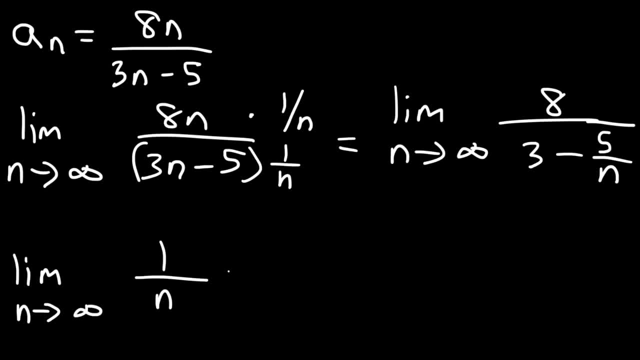 is 0.0123456.. So the number of steps that we can do here is 1 over n. And so what's going to happen? If we take the number and divide it by the number- the constant- we're going to get 1. 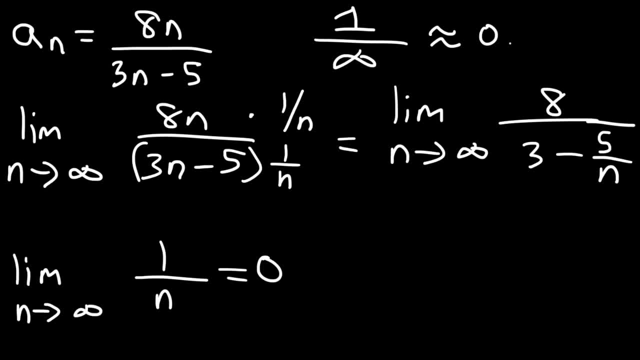 over n. And so if we take the number and divide it by the number- the constant, which is the number that we're going to get- 1 over n, that's going to equal 0. When you take a number like a constant and divide it by a very large number, you're going. 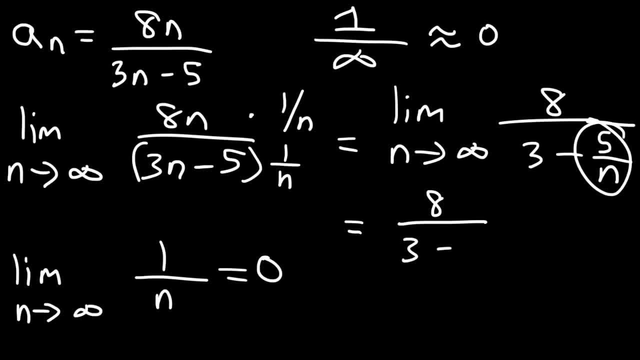 to get a very small number. So, going back to this part of the problem, If we apply the limit expression, we're going to have 8 over 3.. And the limit as n approaches infinity for 5 over n is 0.0123456. 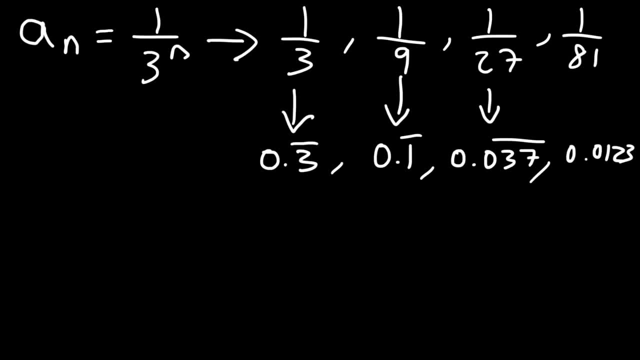 Okay. So notice that as n increases, a sub n is decreasing. In fact, as n approaches infinity, a sub n approaches 0.. So because it's approaching a specific number, we could say that the sequence converges. So we could say that the limit as n approaches infinity. 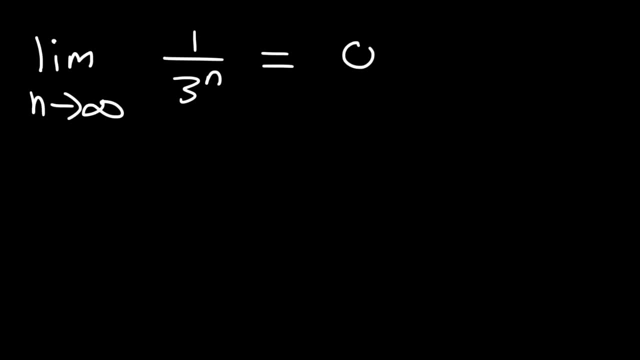 Okay, As n approaches infinity, a sub n over 3 to the n converges to 0.. So the sequence converges And that's the answer. Now let's try another example. So let's say that we have a sub n is equal to 8n divided by 3n minus 5.. 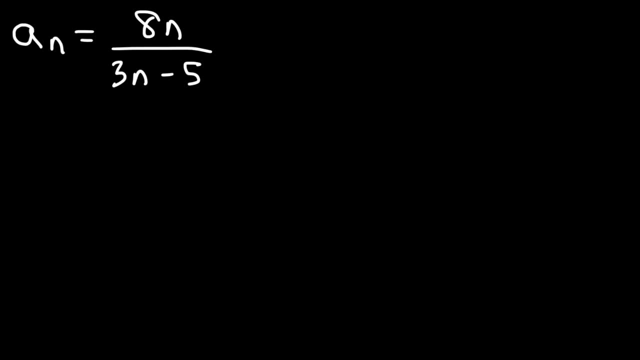 So feel free to pause the video and determine if this sequence converges or if it diverges. So we need to find the limit, Okay, As n approaches infinity for this sequence. So what type of algebraic steps can we do here? What we need to do is multiply the top and the bottom by 1 over n. 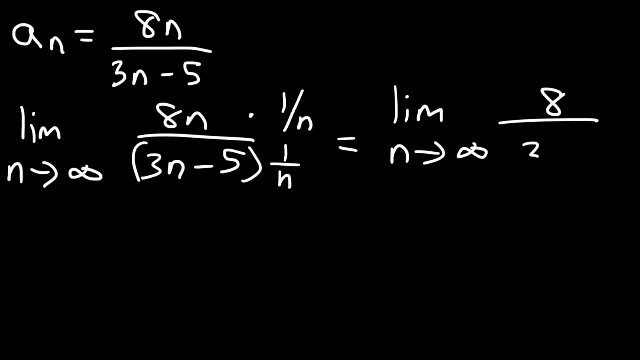 And so we're going to get 8 divided by 3 minus 5 over n. Now it's important to understand that the limit- Okay As n approaches infinity- of some constant like 1 over n, that's going to equal 0.. 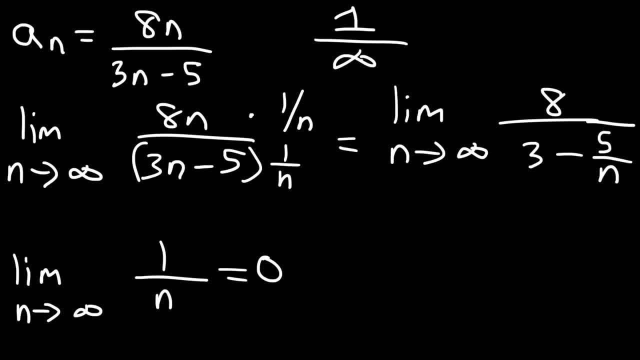 When you take a number like a constant and divide it by a very large number, you're going to get a very small number. So, going back to this part of the problem, if we apply the limit expression, we're going to have 8 over 3.. 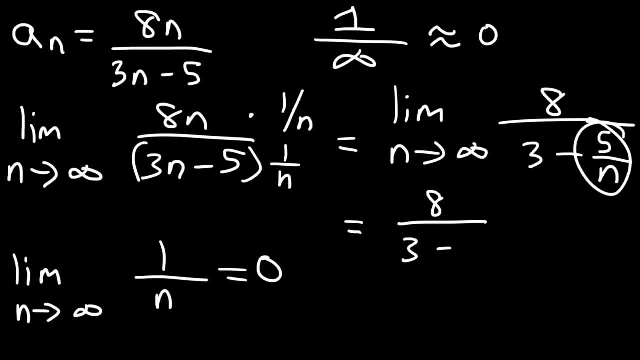 And the limit as n approaches infinity, for 5 over n is 0. Just as 1 over n is 0. So the limit is equal to 8 over 3.. Now, because we have a specific value, we could say that the sequence converges. 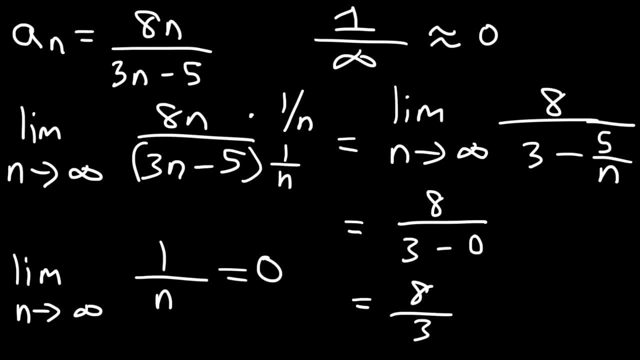 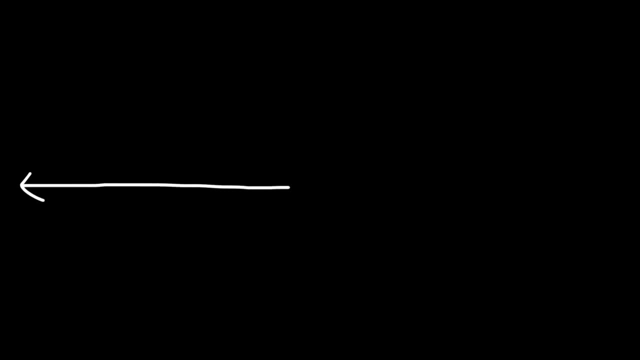 Just says 1 over n is 0.0123456.. So the limit is equal to 8 over 3.. Now, because we have a specific value, we could say that the sequence converges. Now let's get a graphical representation of the function. 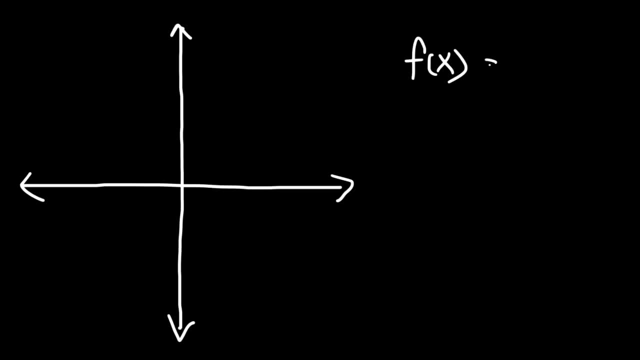 So let's say we have this function: f of x is 8x over 3x minus 5.. This function will have a vertical asymptote at 5 over 3. And it's going to have a horizontal asymptote at 8 over 3.. 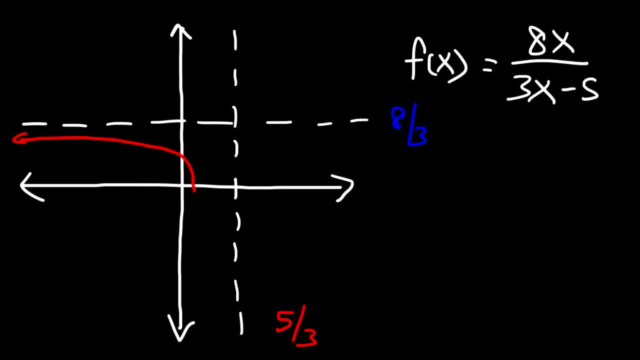 So if we were to graph it, it will look something like this: Now, as x approaches infinity, we would have to follow this curve towards the right And it's going to approach the horizontal asymptote, which is the limit. And so anytime you have a graph that basically converges or follows a horizontal asymptote, it has a limit. 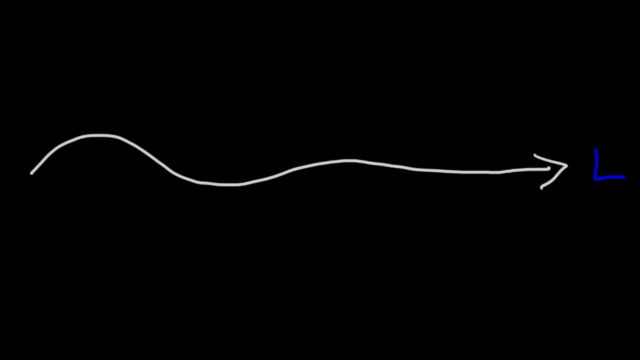 And so you could say that the sequence converges. Now keep in mind, when you're graphing sequences: you don't have a smooth curve. You're dealing with isolated points, So you don't have a smooth curve. So you don't have a smooth curve. 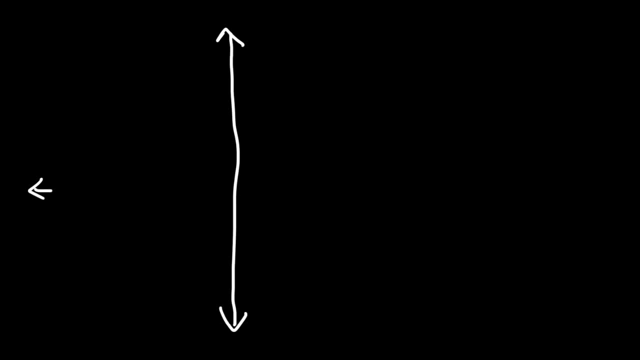 So, for example, if you were to graph that particular sequence, the graph would have: let me draw the vertical asymptote first. It wouldn't be a continuous function. It will have discrete points. So it will look like this: 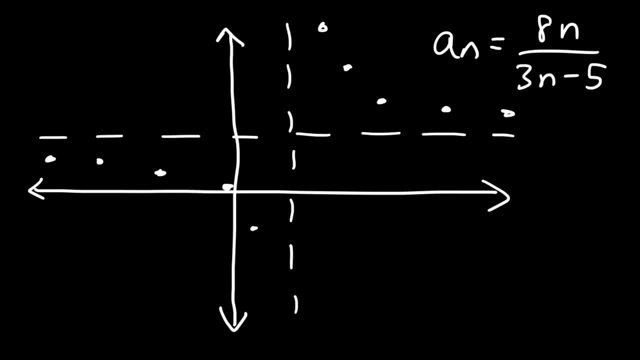 Now, what about a trigonometric function like sine of n? Does it converge or diverge? Well, just as before, let's find the limit as n approaches infinity for sine n. Now what is the answer? 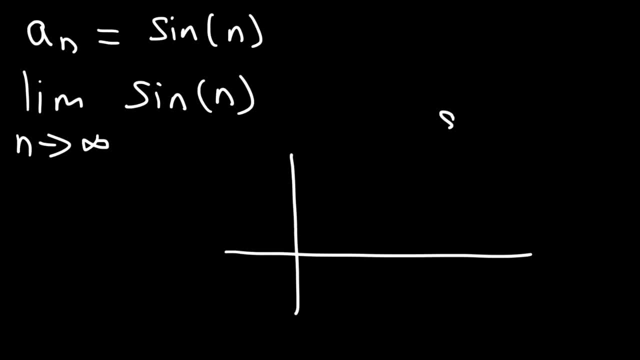 So if we were to draw a graph of sine x, we know that it oscillates between one and negative one. It's a periodic function And so, as you go to the right, it doesn't converge to a specific value. 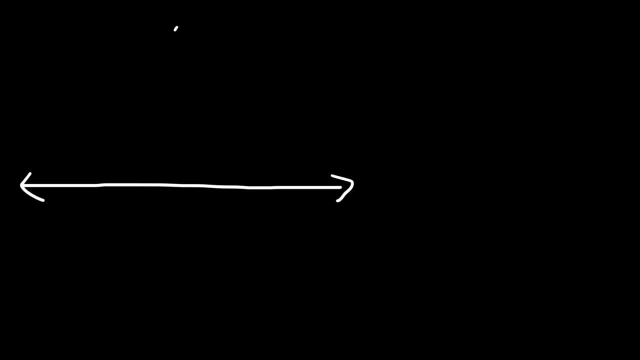 Now let's get a graphical representation of the function. So let's say we have this function: f of x is 8x over 3x minus 5.. Okay, Okay, So this function will have a vertical asymptote at 5 over 3.. 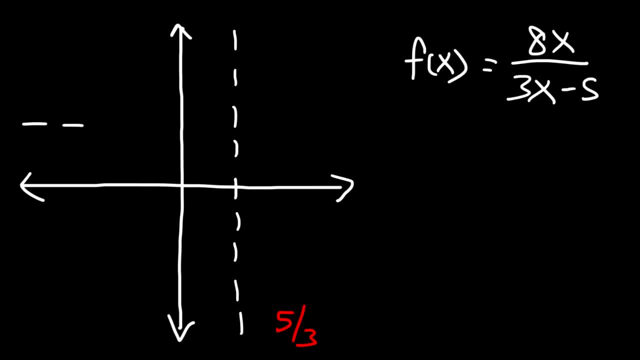 And it's going to have a horizontal asymptote at 8 over 3.. So if we were to graph it, it will look something like this: Okay, Okay, Okay. So if x approaches infinity, we would have to follow this curve towards the right. 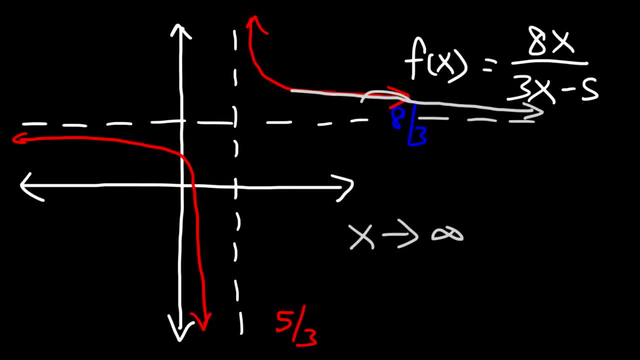 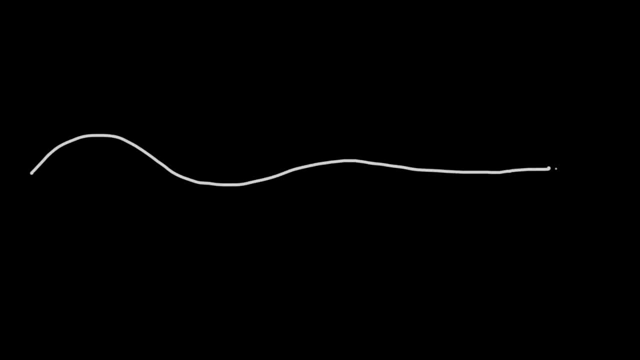 And it's going to approach the horizontal asymptote, which is the limit. And so anytime you have a graph that basically converges or follows a horizontal asymptote, it has a limit, And so you could say that the sequence converges. Now keep in mind, when you're graphing sequences, you don't have a smooth curve. 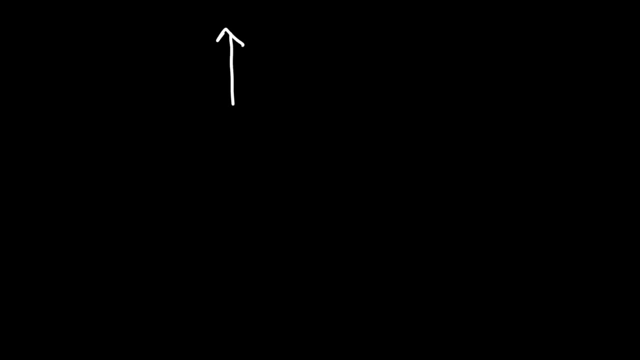 You're dealing with isolated points. So, for example, if you were to graph that particular sequence, the graph would have – let me draw the vertical asymptote first: It wouldn't be a continuous function, It will have discrete points. So it will look like this: 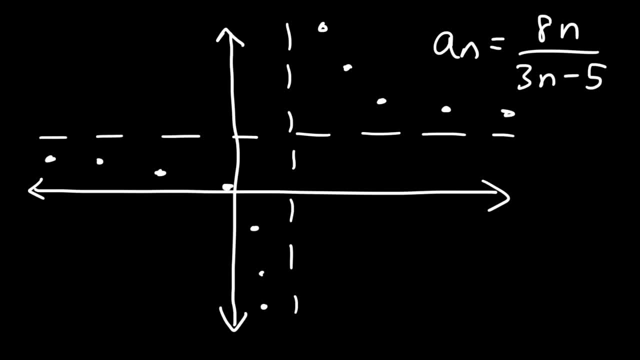 Okay, Okay, Okay, Okay. So just keep that in mind. Now, what about a trigonometric function like sine of n? Does it converge or diverge? Well, just as before, let's find the limit as n approaches infinity for sine n. 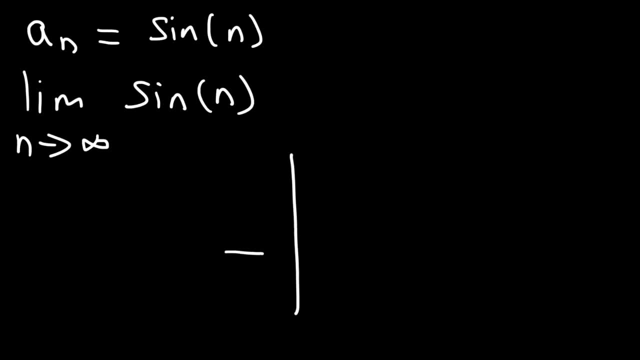 Now, what is the answer? So if we were to draw a graph of sine x, Okay, Okay, Okay. So we know that it oscillates between 1 and negative 1.. It's a periodic function And so, as you go to the right, it doesn't converge to a specific value. 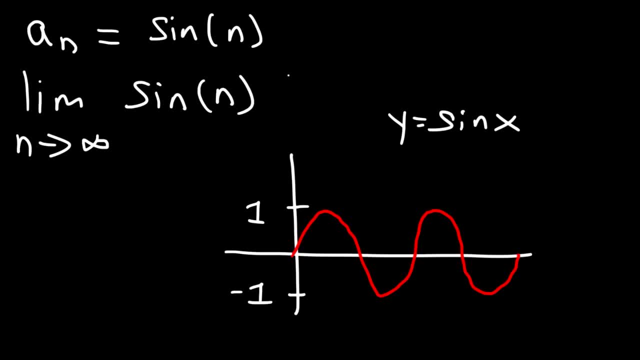 It's always oscillating between negative, one and one. So therefore the limit as n approaches infinity, it does not exist, It doesn't go to infinity, It doesn't go to zero, It just keeps oscillating. So we could say that this particular sequence, it diverges. 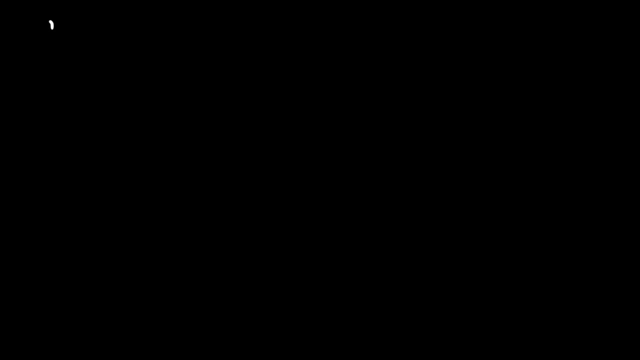 It doesn't converge. Now let's move on to our next example. a sub n is equal to cosine one over n. So what about that sequence? Will it converge or diverge? So take a minute and work on that example. So what is the limit as n approaches infinity of cosine one over n? 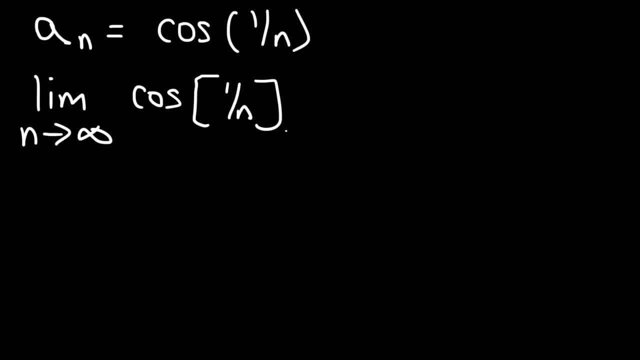 Now we know the limit, as n approaches infinity, for one over n, That is zero, And so this becomes cosine zero, And cosine zero is equal to a specific value, which is one. So therefore the limit, I mean not the limit, but the sequence. 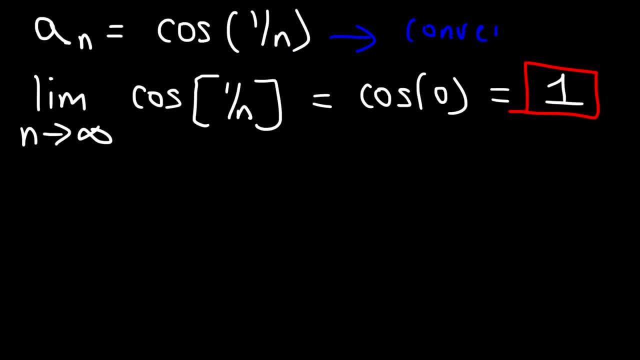 the sequence itself converges Because the limit is equal to a specific value. Now take out your graphing calculator And let's graph the function cosine one over x. Let's say this is one and negative one, And somewhere over here it's positive one. 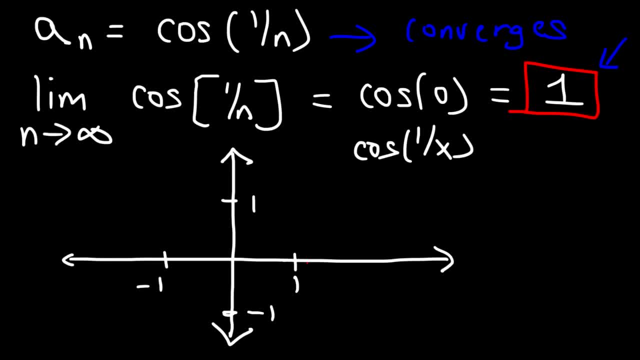 So just below one the graph will oscillate a lot. My graph is not perfect, but it's just going to oscillate rapidly And then it's going to follow the horizontal asymptote at one. So that's the general shape of this graph. 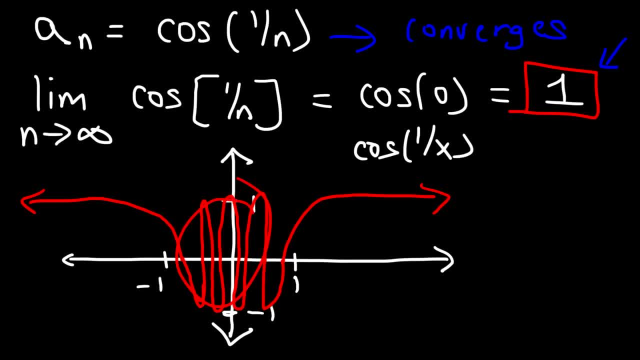 If you graph it, you may not be able to see this. It's oscillating so much next to zero that it just looks like one big blur. But the important part of what you want to keep in mind is that, all the way to the right, 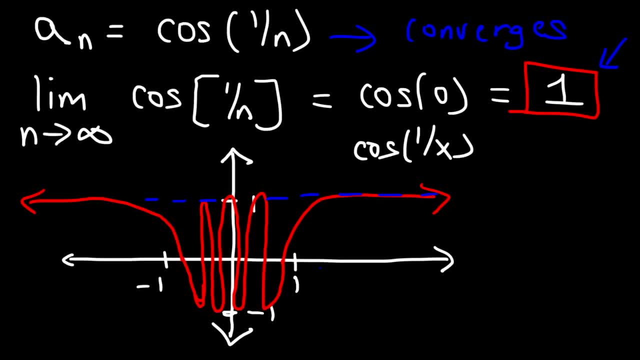 it follows the horizontal asymptote And so whenever you see that in a graph, you know that the sequence converges. It converges at one. So sometimes, if you're not sure what, the answer is: just graph the sequence. 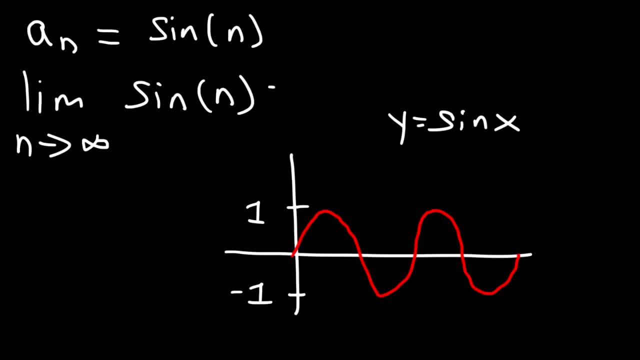 It's always oscillating between negative 1 and 1.. So therefore, the limit as n approaches infinity, it does not exist, It doesn't go to infinity, It doesn't go to 0.. It just keeps oscillating. So we could say that this particular sequence. 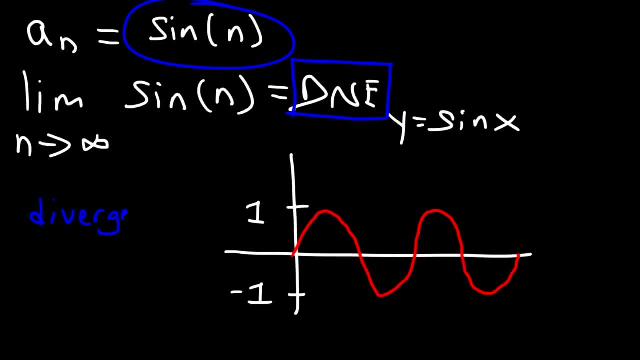 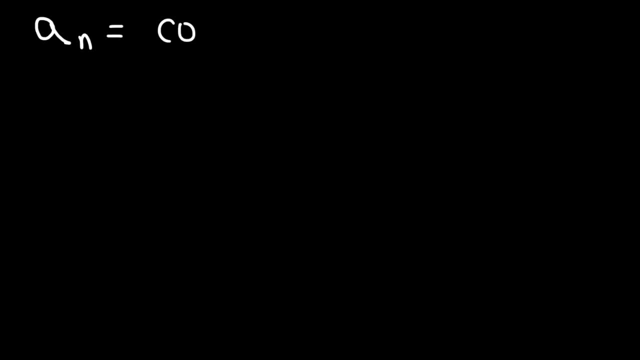 it diverges, It doesn't converge. Now let's move on to our next example. a sub n is equal to cosine 1 over n. So what about that sequence? Will it converge or diverge? So take a minute and work on that example. So what is the limit as n approaches infinity of cosine 1? 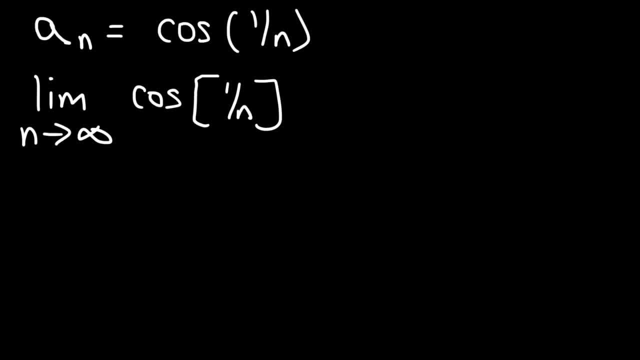 over n. Now we know the limit: as n approaches infinity, for 1 over n, that is 0. And so this becomes cosine 0.. And cosine 0 is equal to a specific value, which is 1.. So therefore, the limit- I mean not the limit, but the sequence, the sequence itself- converges. 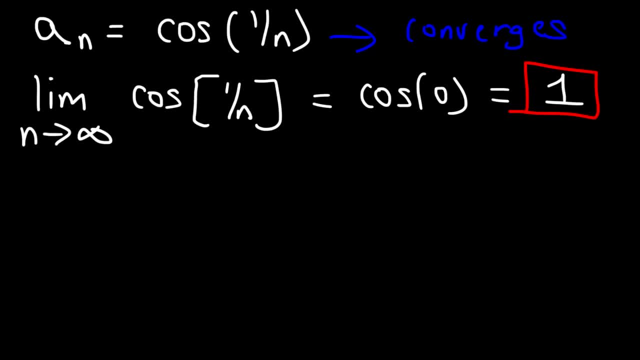 because the limit is equal to a specific value. Now take out your graphing calculator And let's graph the function cosine 1 over x. Let's say this is 1 and negative 1 and somewhere over here it's positive 1.. So just below 1, the graph will oscillate a lot. My 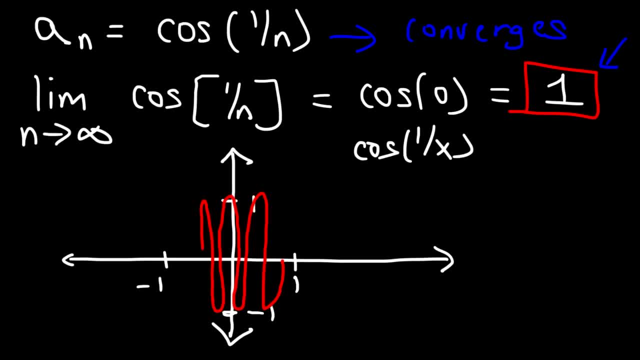 graph is not perfect, but it's just going to oscillate rapidly. It's going to follow the horizontal asymptote at 1.. So that's the general shape of this graph. If you graph it, you may not be able to see this. It's oscillating so much. next, 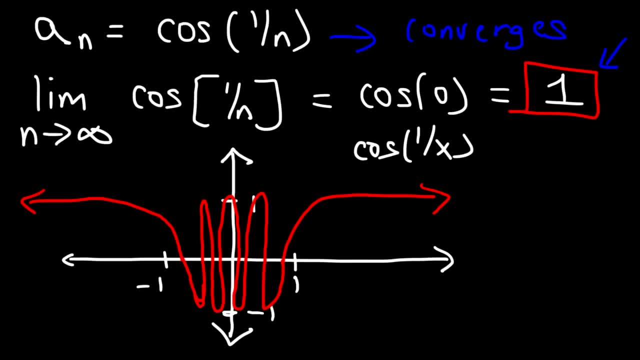 to 0 that it just looks like one big blur. But the important part of what you want to keep in mind is that all the way to the right, it follows the horizontal asymptote, And so if you see that in a graph, you know that the sequence converges. It converges at 1.. 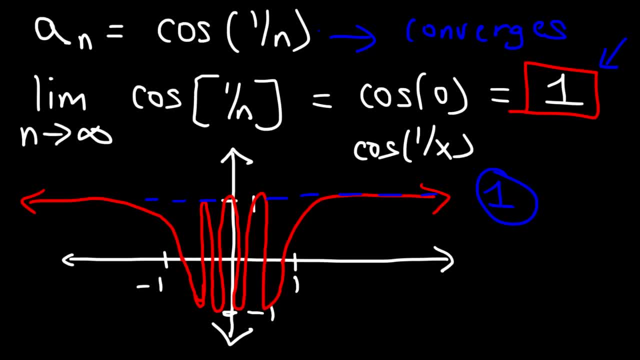 So sometimes, if you're not sure what the answer is, just graph the sequence And then see if it approaches a horizontal asymptote. If it does, then you know the sequence converges. If it does not, you know it diverges. 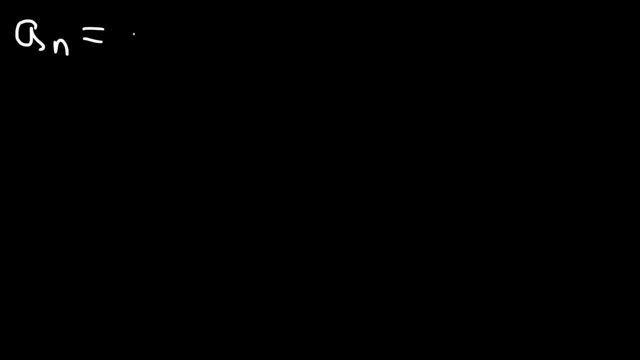 Here's another example that involves a trigonometric function. Consider the sequence sine n, divided by n. So go ahead and determine if this sequence converges or diverges. So if you had to take a good guess, what would you say? Well, we know that sine, it varies between negative 1 to 1.. And it's divided by n, So 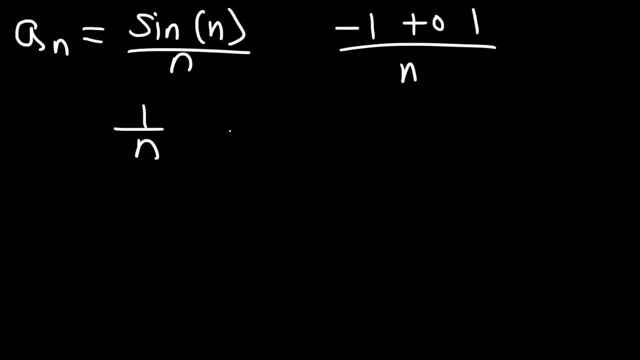 whenever you have a constant, let's say 1 over n, as n approaches infinity, this will become 0. The same is true for negative 1 over n. Negative 1 divided by a very large number is approximately 0. So we can see that this particular sequence is going to converge. 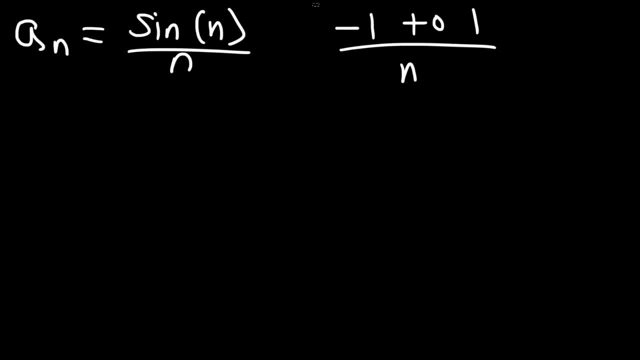 But how do we show it? So, let's say, if you have a free response question and you need to show your work, How can we show that the sequence converges? This is when you need to use the squeeze theorem. Now, just to review, the basic idea behind the squeeze theorem is you have, let's say, 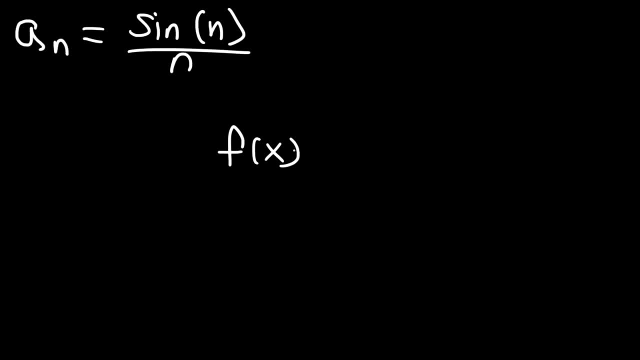 some function. Let's call it f of x. Now let's say it's between g of x and h of x. Now the limit as x approaches, let's say infinity. for g of x, let's say it's equal to some limit L. 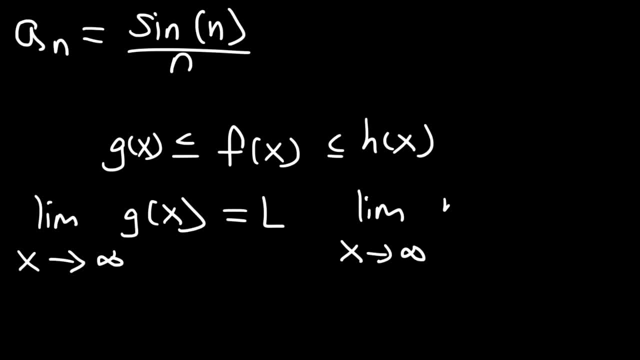 And the limit as x approaches infinity for h of x is also L. So if g and h have the same limit, then the function in the middle according to the squeeze theorem should also have the same limit. So the limit as x approaches infinity for f of x must also be L, because f is between. 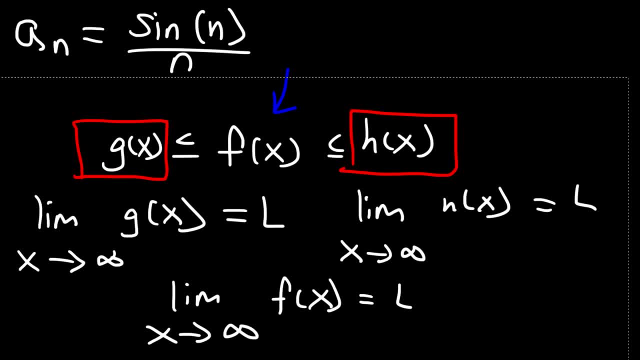 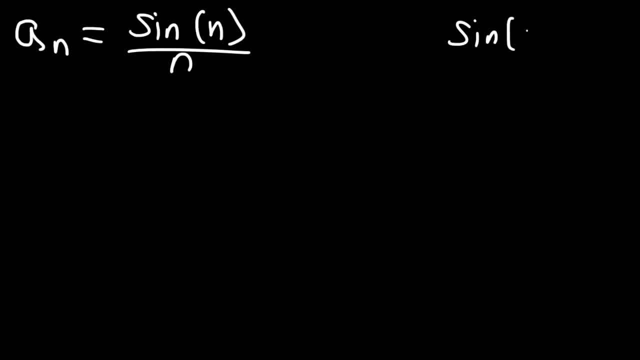 g and h, And so that's the theorem that we need to use here. Now we know that sine it varies between negative 1 and 1.. Now if we divide all three sides of the inequality by n, we're going to get this expression. 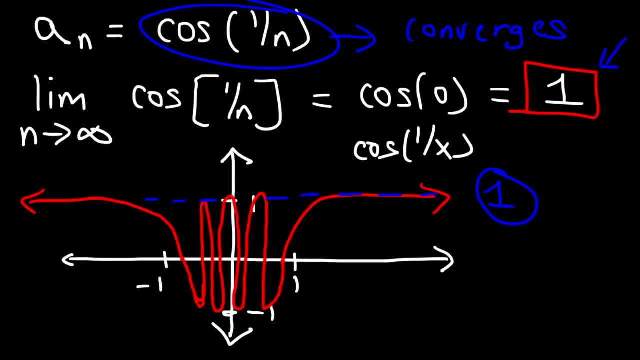 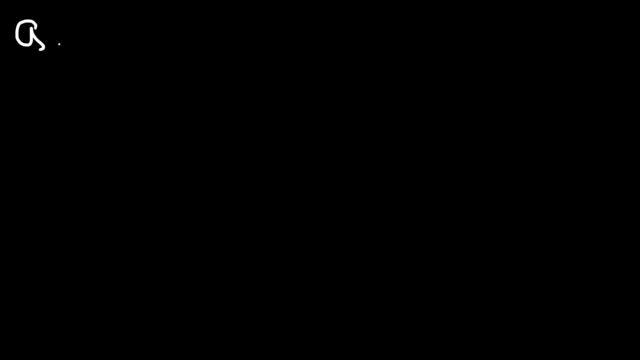 And then see if it approaches a horizontal asymptote. If it does, then you know the sequence converges. If it does not, you know it diverges. Here's another example that involves a trigonometric function. Consider the sequence sine n divided by n. 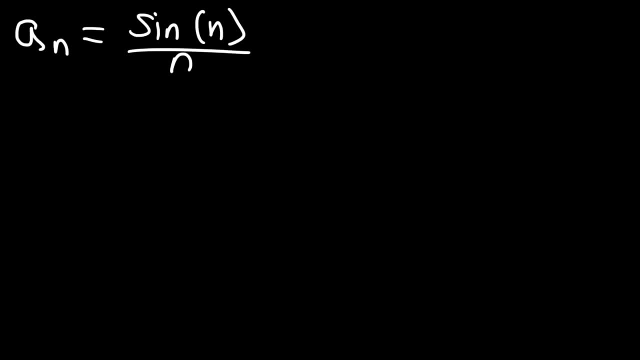 So go ahead and determine if this sequence converges or diverges. So if you had to take a good guess, what would you say? Well, we know that, sine, it varies between negative one to one And it's divided by n. 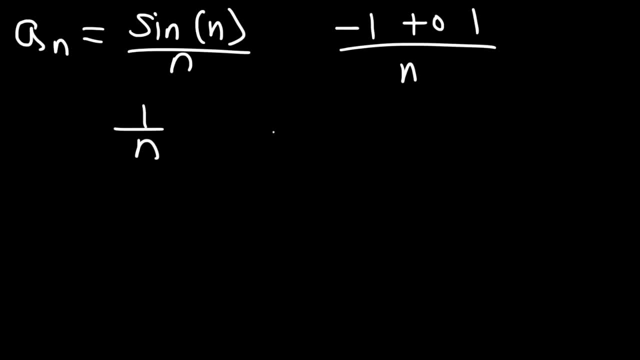 So whenever you have a constant, let's say one over n, as n approaches infinity, this will become zero. The same is true for negative one over n. Negative one divided by a very large number is approximately zero. So we can see that this particular sequence is going to converge. 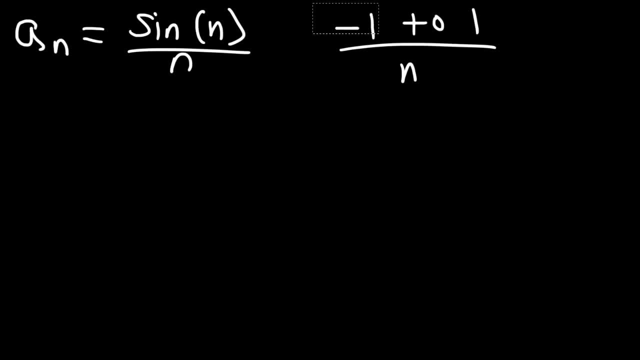 But how do we show it? So, let's say, if you have a free response question and you need to show your work, How can we show that the sequence converges? This is when you need to use the squeeze theorem. Now just to review the basic idea behind the squeeze theorem: 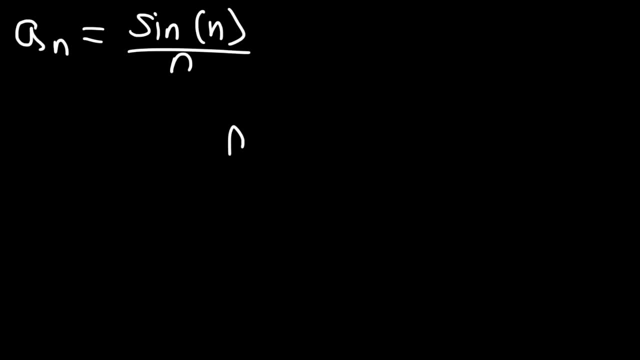 is. you have, let's say, some function. let's call it f. Now let's say it's between g and h. Now the limit as x approaches, let's say infinity for g, So let's say it's equal to some limit L. 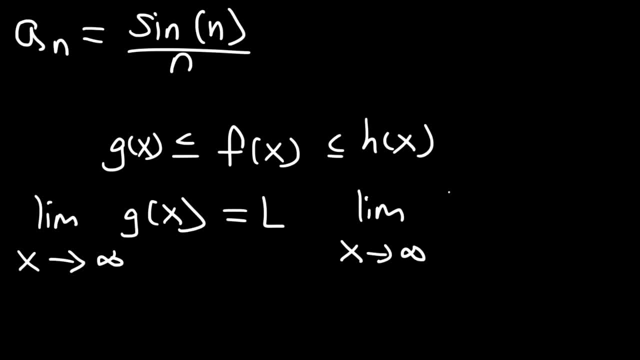 And the limit as x approaches infinity for h is also L. So if g and h have the same limit, then the function in the middle according to the squeeze theorem should also have the same limit. So the limit as x approaches infinity for f must also be L. 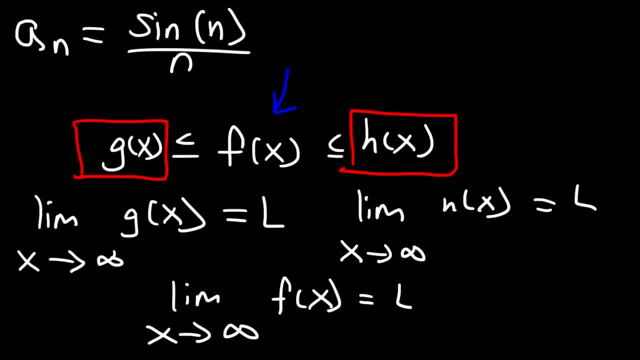 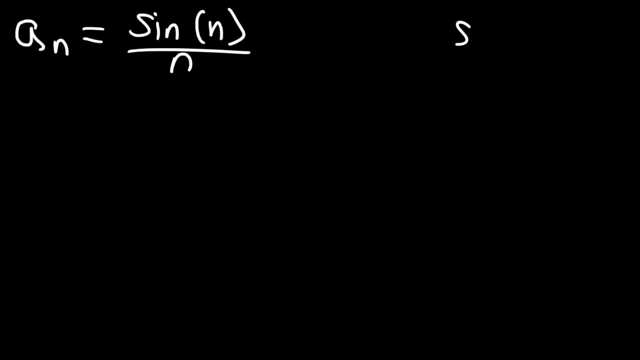 Because f is between g and h, And so that's the theorem that we need to use here. Now we know that sine it varies between negative one and one. Now if we divide all three sides of the inequality by n, we're going to get this expression. 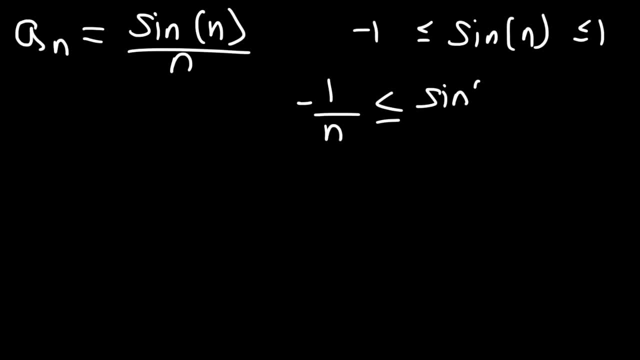 Negative: one over n is less than or equal to sine n over n, which is less than or equal to one over n. So now this expression is in a form in which we could use the squeeze theorem. So let's identify the limit as n approaches infinity. 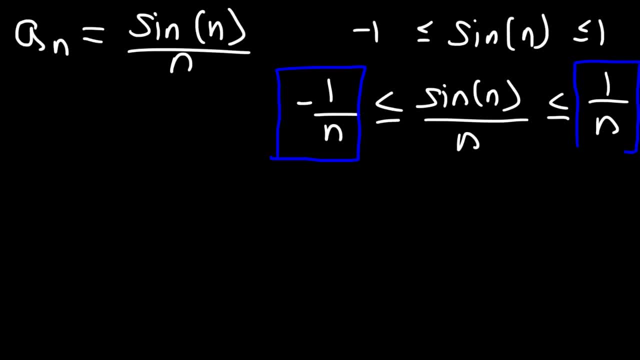 for these two parts Of this inequality. So the limit as n approaches infinity for negative one over n, that is going to be zero. And the limit as n approaches infinity for positive one over n. 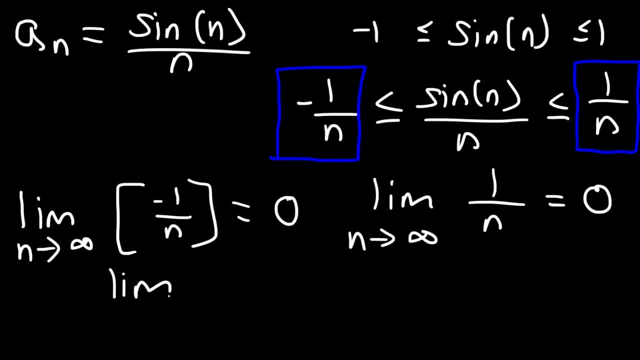 as we know, is also zero. So therefore, according to the squeeze theorem, the limit as n approaches infinity for sine n over n must also be zero, And so therefore, we could say that this sequence converges. 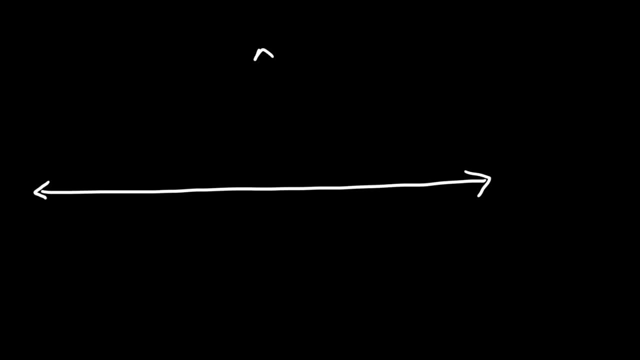 Now let's draw a graph. So let's graph the function sine x divided by x. So plug this in your graphing calculator. At one you should have an open circle or a hole. Now the graph may not show the hole. 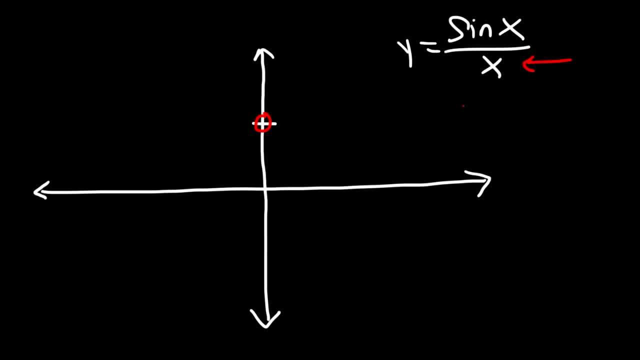 but you know that x cannot be zero, Otherwise the function will be undefined. But everywhere else let's say: if x is point one and sine is point one, where it's in radian mode, that's going to equal one. 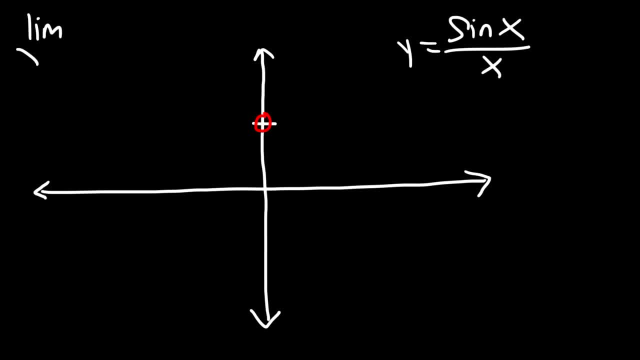 The limit as x approaches zero for sine x over x is one. These are one of the limits that you just need to know, So we should have a hole, But then, if you continue to graph it, it should look something like this: 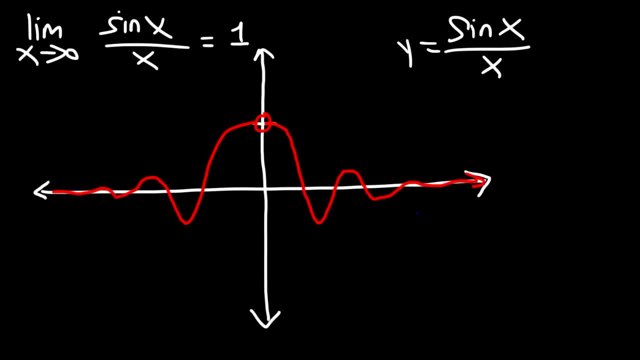 And so, as you can see, as you follow the curve all the way to the right notice, that it follows the x-axis, Which means the horizontal asymptote is following is y equals zero, So that's why the limit 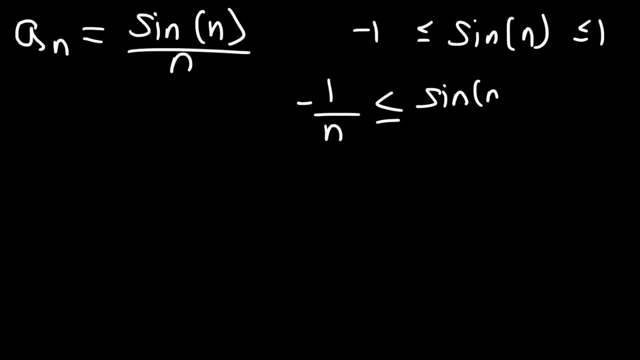 Negative, 1 over n is less than or equal to sine n over n, which is less than or equal to 1 over n. So now this expression is in a form in which we could use the squeeze theorem. So let's identify the limit, as n approaches infinity, for these two parts of this inequality. 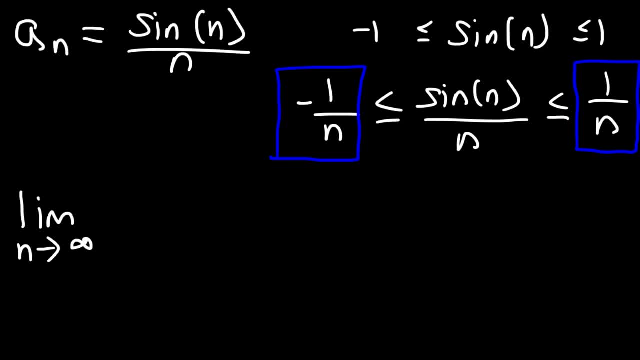 So the limit as n approaches infinity is 1 over n. So if we find n approaches infinity for negative 1 over n, that is going to be 0.. And the limit as n approaches infinity for positive 1 over n, as we know, is also 0.. 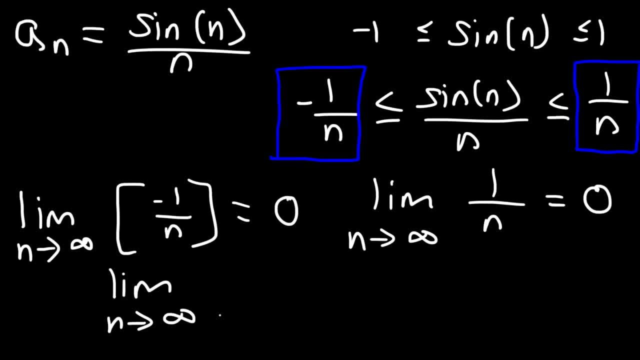 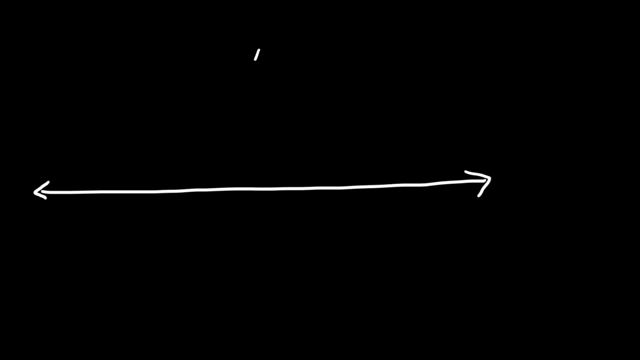 So therefore, according to the squeeze theorem, the limit as n approaches infinity, for sine n over n must also be 0.. And so therefore we could say that this sequence converges. Now let's draw a graph. so let's graph the function sine x divided by x. So 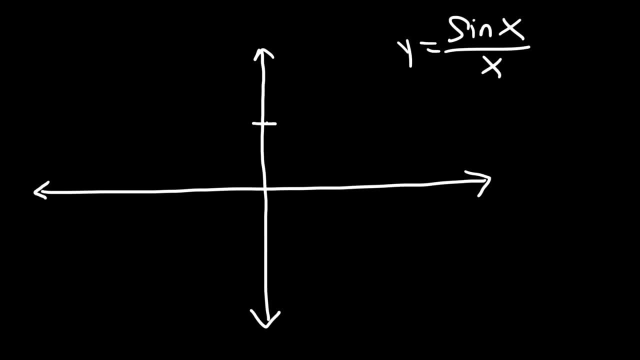 plug this in your graphing calculator At 1, you should have an open circle or hole. Now the graph may not show the hole, but you know that x cannot be 0, otherwise the function will be undefined. But everywhere else let's say: if x is 0.1 and sine is 0.1, where it's. 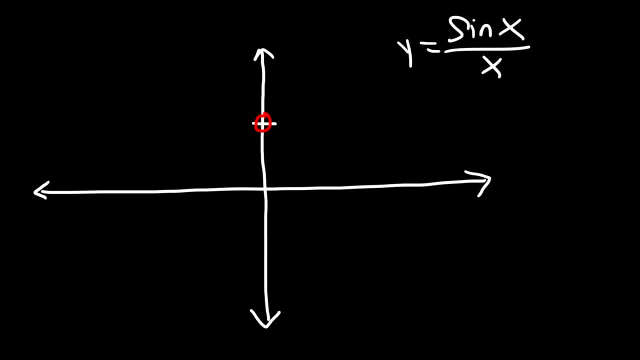 in radian mode that's going to equal 1.. The limit as x approaches 0 for sine x over x is 1.. These are one of the limits that you just need to know. So we should have a hole. but then, if you continue to graph it, it should look something like this: 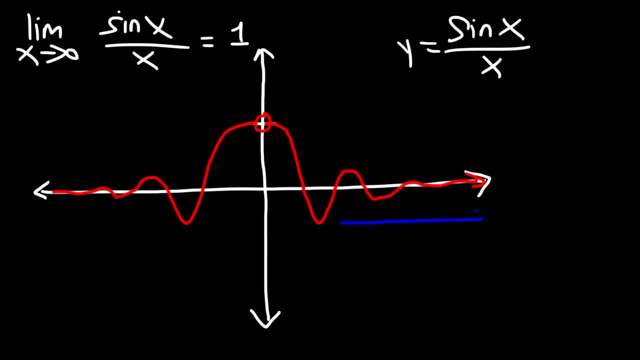 And so, as you can see, as you follow the curve all the way to the right notice, that it follows the x-axis, which means the horizontal asymptote it's following is: y equals 0.. So that's why the limit is equal to 0.. It converges to 0.. 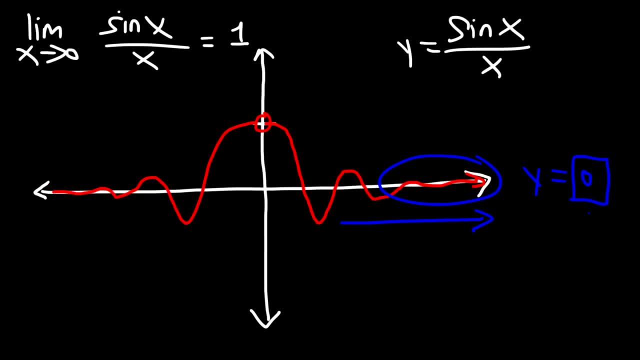 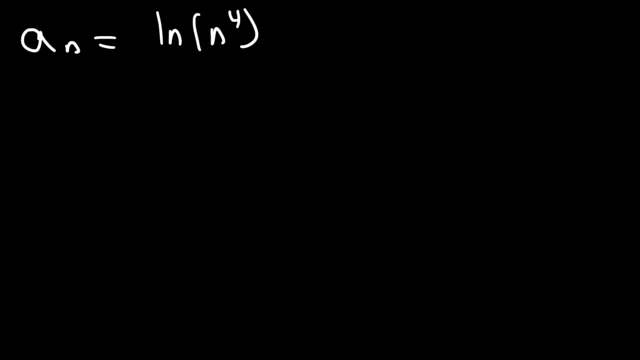 is equal to zero, It converges to zero. Try this one: The natural log of n to the fourth over 5n. So will the sequence converge or diverge? So what is the limit as n approaches infinity? 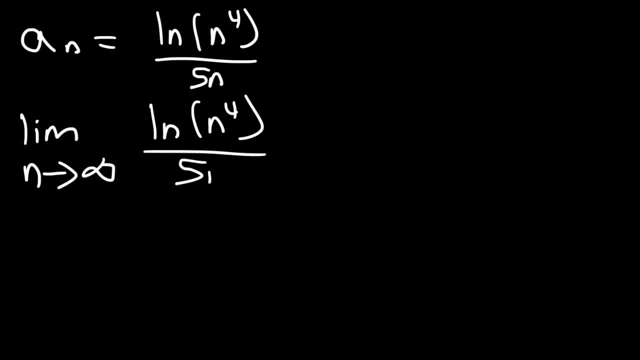 for the natural log of n to the fourth, divided by 5n. Well, we need to use the L'Hopital's Rule to get the answer, But before we do that, let's take the 4 and move it to the front. 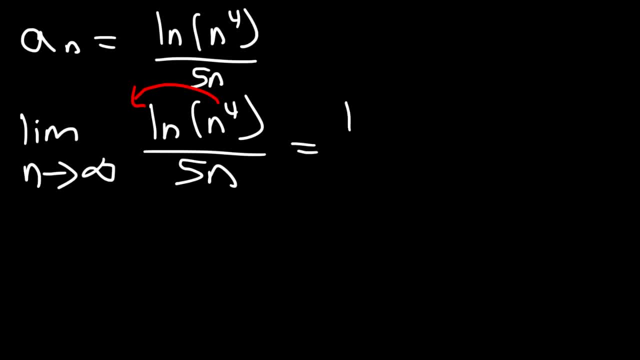 So we can employ a property of logs. So we have the limit as n approaches infinity, and then 4 times the natural log of n divided by 5n. Now, in this form, use L'Hopital's Rule. 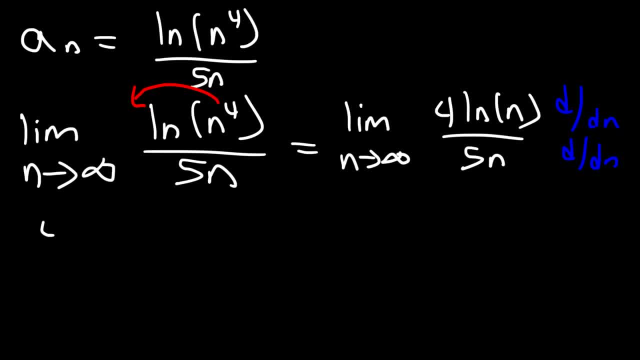 So the derivative of the numerator, the derivative of ln, n, is 1 over n- Let me rewrite the limit expression first- And the derivative of 5n is simply 5.. So what we now have is- I'm going to move the constant 4 over 5.. 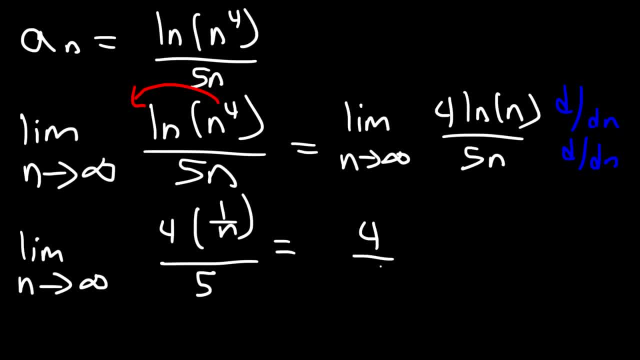 to the front. So this is equal to 4 over 5. times the limit as n approaches infinity, for 1 over n, Which we know to be zero. So it's 4 over 5. times zero. 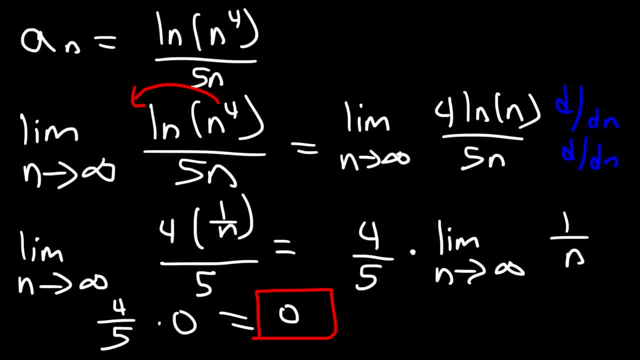 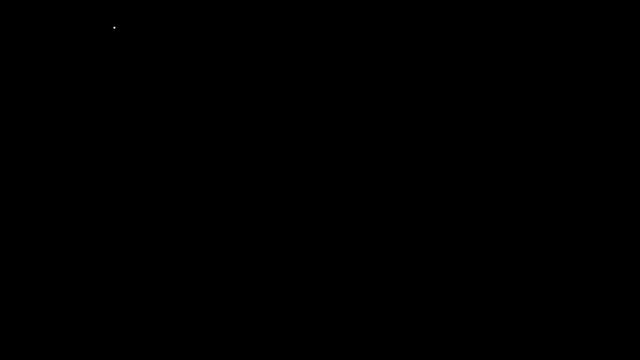 which is zero. So therefore, the sequence converges. Let's try another trigonometric function, This time n times sine, raised to the 1 over n. So what do you think? Will this sequence converge or diverge? 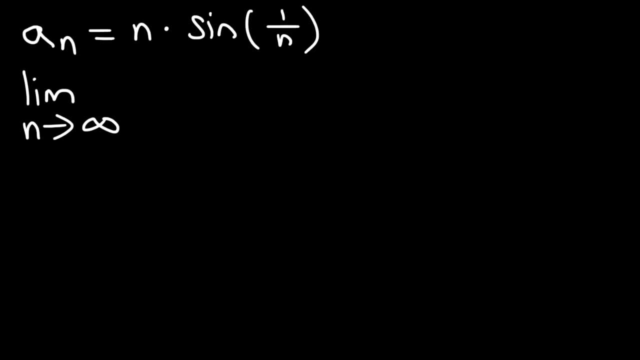 So what is the limit? as n approaches infinity, n times sine 1 over n. So how can we find the answer? We need to use L'Hopital's Rule, But right now it's not in the appropriate form. 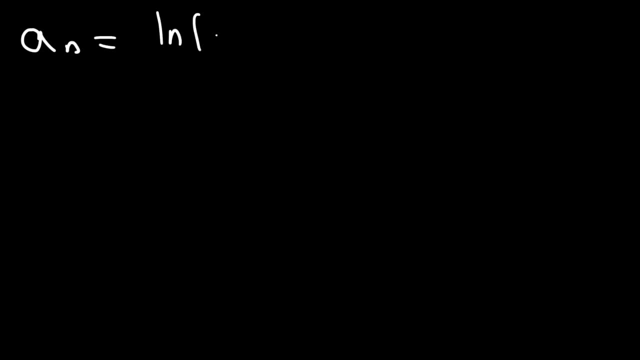 Let's try this one: The natural log of n to the 4th over 5n. So will the sequence converge or diverge? So what is the limit, as n approaches infinity, for the natural log of n to the 4th divided? 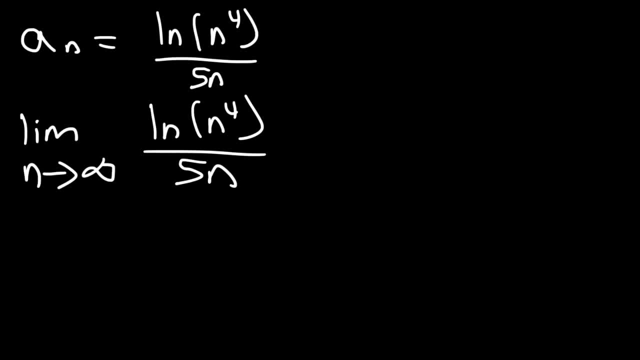 by 5n. Well, we need to use the L'Hopital's rule to get the answer. but before we do that, let's take the 4 and move it to the front, So we can employ the L'Hopital's rule to get the. 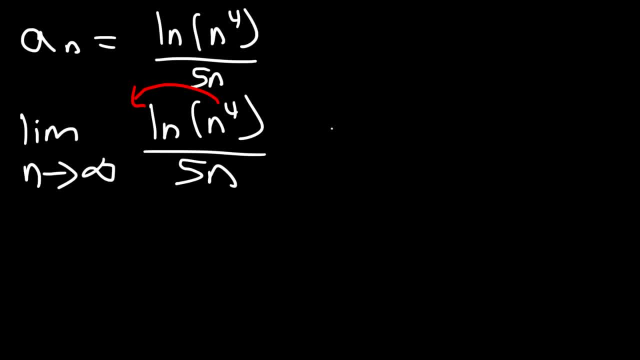 answer. but before we do that, let's take the 4 and move it to the front, So we can, So we can employ a property of logs. So we have the limit as n approaches infinity, and then 4 times the natural log of n divided by 5n. 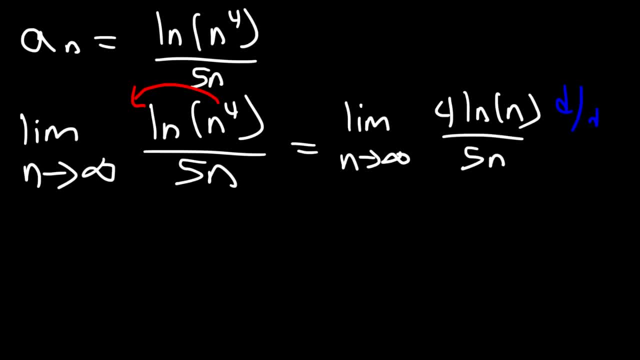 Now in this form, use L'Hopital's rule. So the derivative of the numerator, the derivative of ln, n, is 1 over n. Let me rewrite the limit expression first. And the derivative of 5n is simply 5.. 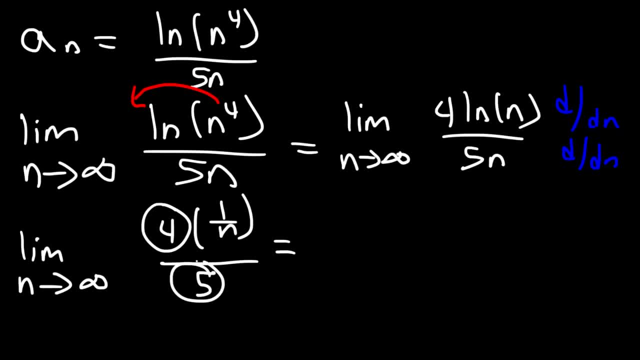 So what we now have is I'm going to move the constant 4 over 5 to the front, So this is equal to 4 over 5 times the limit, as n approaches infinity, for 1 over n, which we know to be 0.. 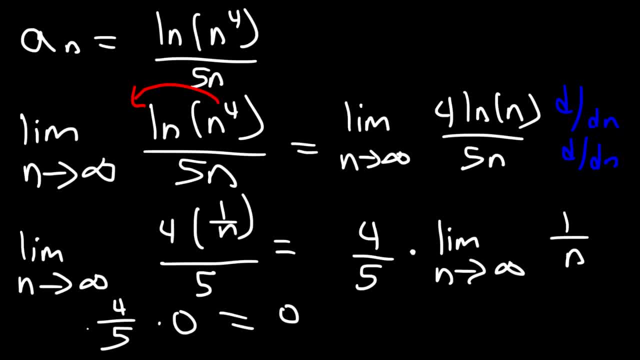 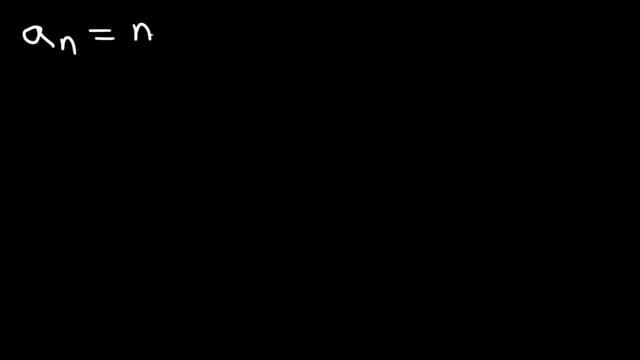 So it's 4 over 5 times 0, which is 0.. So therefore, the sequence converges. Let's try another trigonometric function, This time n times sine, raised to the 1 over n. So what do you think? Will this sequence converge or diverge? 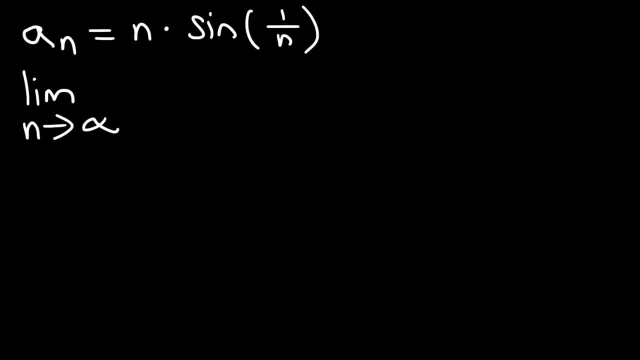 So what is the limit as n approaches infinity, n times sine 1 over n. So how can we find the answer? We need to use the limit expression, We need to use L'Hopital's rule, But right now it's not in the appropriate form. 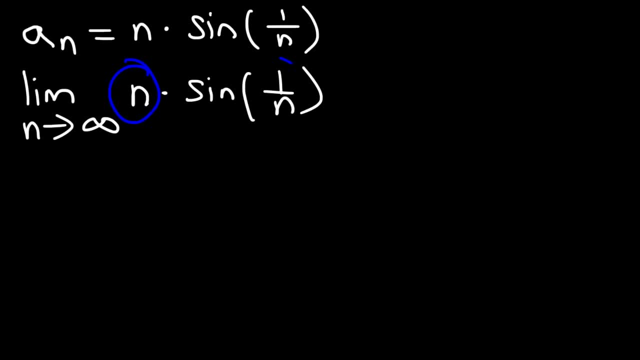 So we need a fraction. We have basically two parts multiplied to each other. Somehow we have to turn this situation from multiplication to division, And here's how you can do it. You need to know that n is the same as 1 divided by 1 over n. 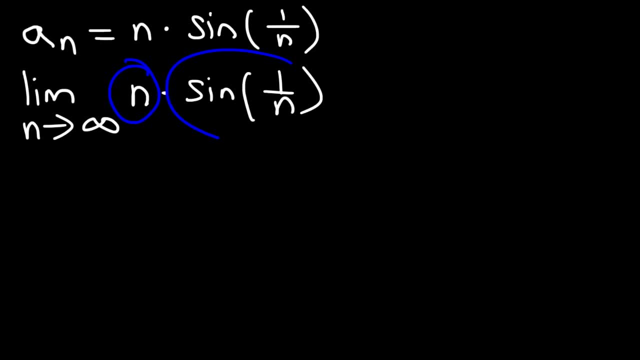 So we need a fraction. We have basically two parts multiplied to each other. Somehow we have to turn this situation from multiplication to division, And here's how you can do it. You need to know that n. 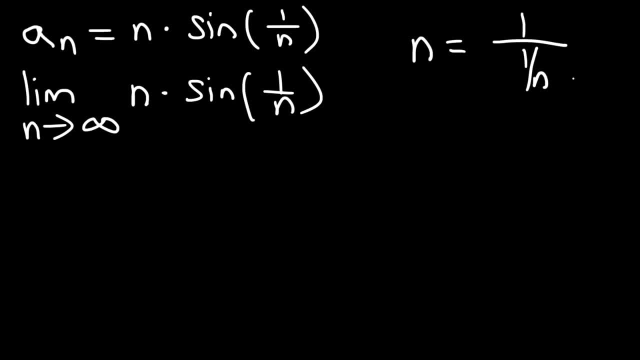 is the same as 1. divided by 1 over n. So replace an n with this fraction. We're going to get the limit as n approaches infinity, sine .1 over n. divided by 1 over n. 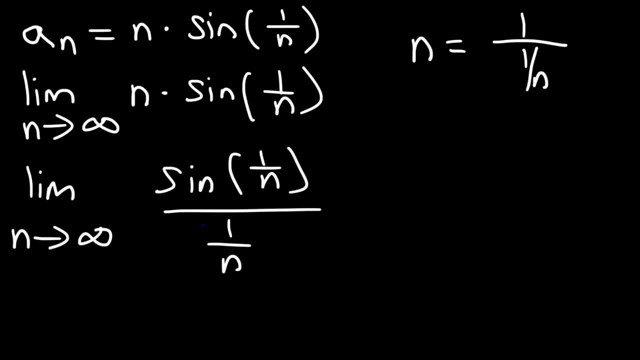 So now we can use L'Hopital's Rule. So let's differentiate the numerator and the denominator, The derivative of 1 over n. if you use the Power Rule first you need to rewrite it as n to the minus 1.. 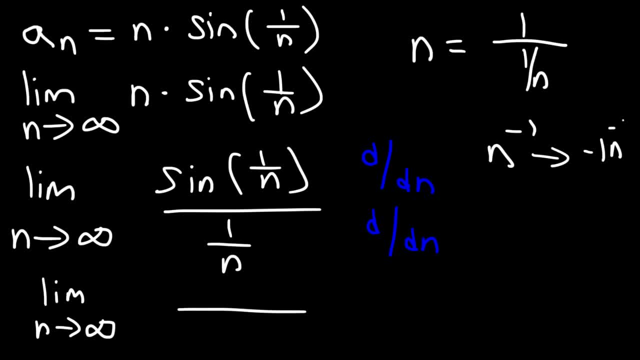 And so it becomes negative 1.. n to the negative 2. And then, rewriting it again, it's negative 1 over n, squared. Now, the derivative of sine is cosine, And, based on the Chain Rule, we need to keep the inside part the same. 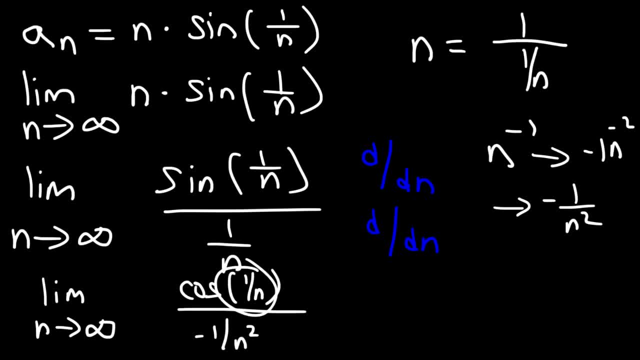 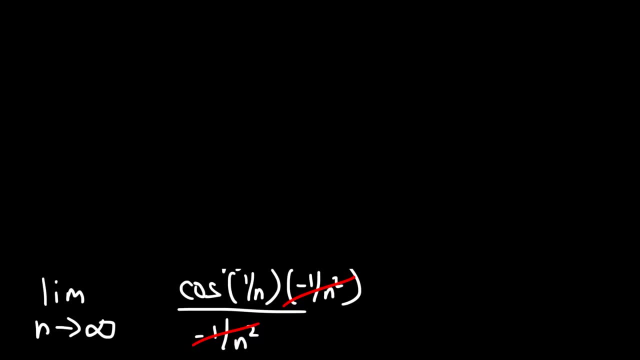 And then differentiate the nested function 1 over n, which is negative .1 over n squared, And so we could cancel negative 1 over n squared, And so what we now have is that the limit. 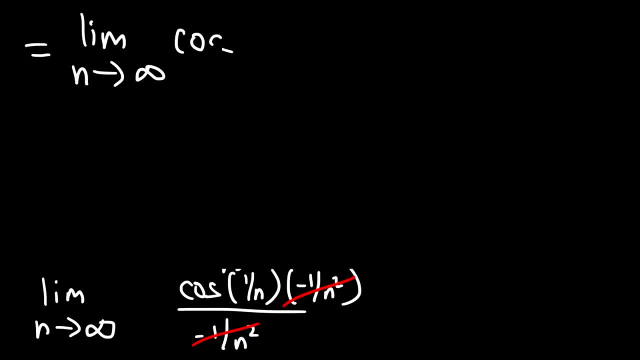 as n approaches infinity, and we're left over with cosine 1 over n. Now for 1 over n. as n approaches infinity, we know that's going to be 0. And so this becomes cosine of 0.. 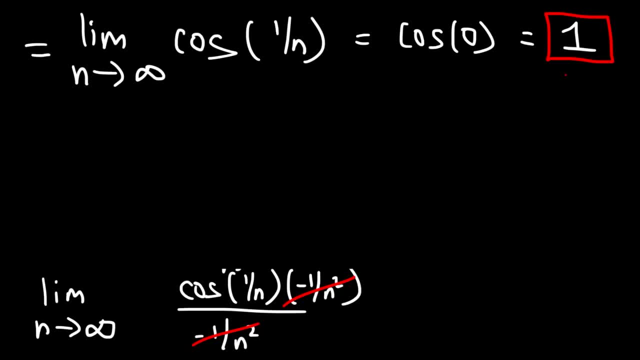 which is equal to 1.. So therefore, this sequence converges. Now let's try a problem with factorials. Let's say we have n plus 1 factorial over n factorial, So will the sequence converge. 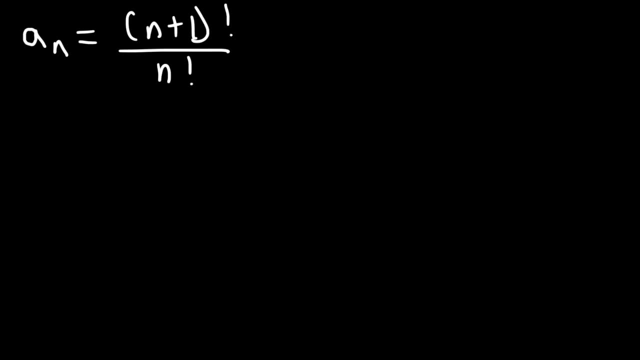 or diverge. In this case you need to know how to simplify factorials. So let's say, if we have a factorial, 8 times 7, times 6. times 5. all the way to 1.. 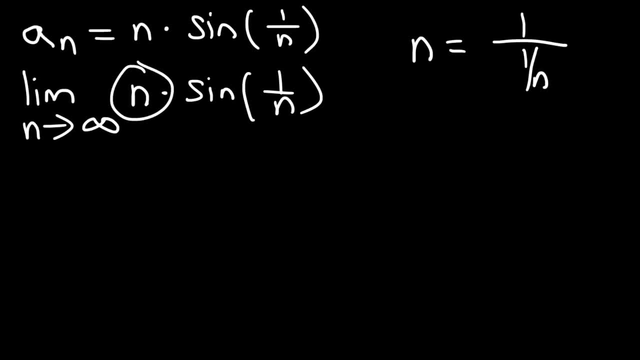 So replace an n with this fraction. We're going to get the limit as n approaches infinity, sine: 1 over n, divided by 1 over n. So now we can use L'Hopital's rule. So let's differentiate the numerator and the denominator. 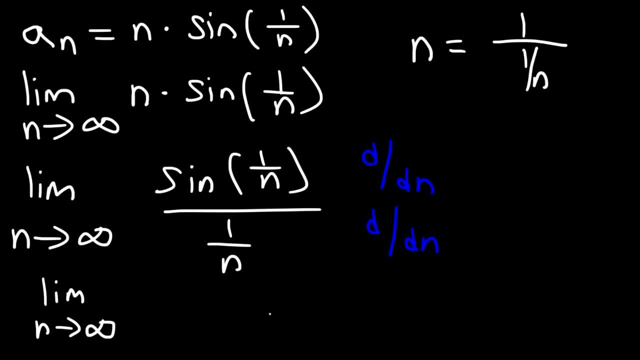 So let's differentiate the numerator and the denominator, The derivative of 1 over n. if you use the power rule first, you need to rewrite it as n to the minus 1.. And so it becomes negative 1, n to the negative 2.. 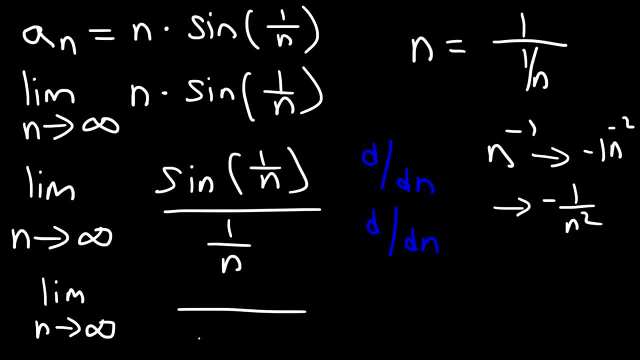 And then rewriting it again, it's negative: 1 over n squared. Now the derivative of sine is cosine And, based on the chain rule, we need to keep the inside part the same And then differentiate the nested function 1 over n. 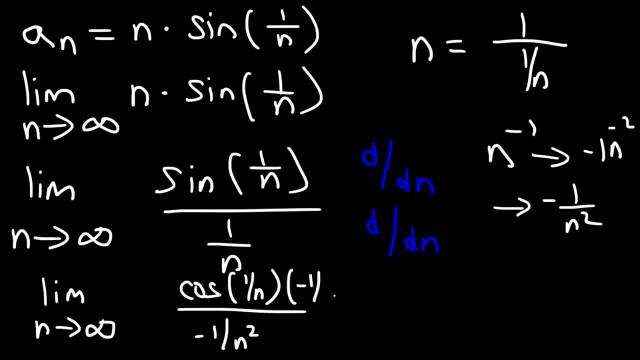 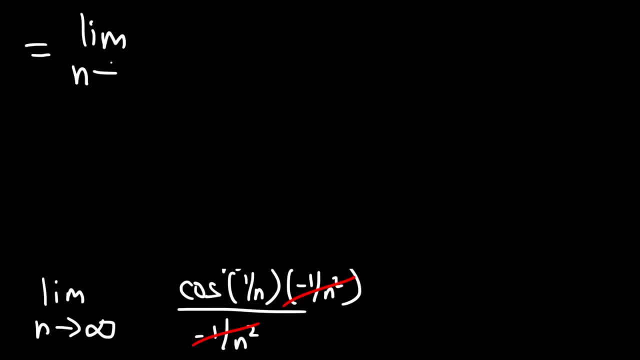 which is negative 1 over n squared, And so we could cancel negative 1 over n squared. And so what we now have is that the limit as n approaches infinity and we're left over with cosine 1 over n. Now for 1 over n. as n approaches infinity, we know that's going to be 0.. 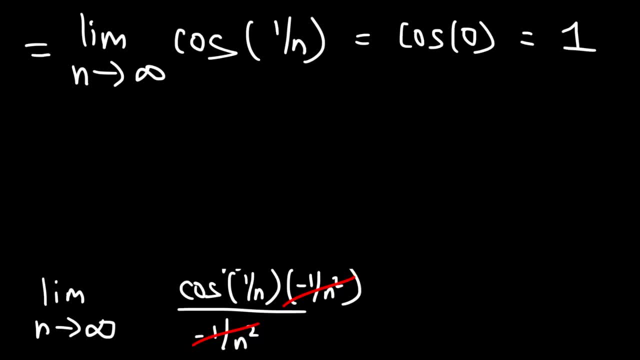 And so this becomes cosine of 0, which is equal to 1.. So therefore, this sequence converges. Now let's try a problem with factorials. Let's say we have a problem with factorials. Let's say we have n plus 1 factorial over n factorial. 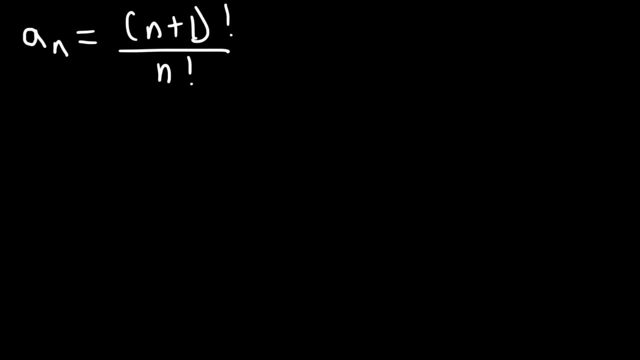 So will the sequence converge or diverge? In this case, you need to know how to simplify factorials. So let's say, if we have a factorial, This is basically 8 times 7 times, 6 times 5,, all the way to 1.. 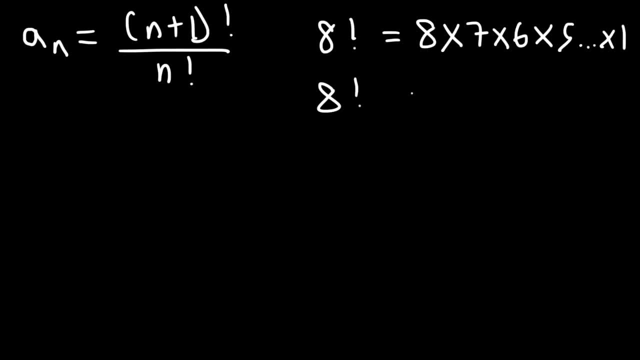 That's a factorial. Now you can also write a factorial as 8 times 7 factorial, Because 7 factorial is basically 7 times 6 times 5 times 4,, all the way to 1.. Now this is the way in which we want to simplify a situation like this. 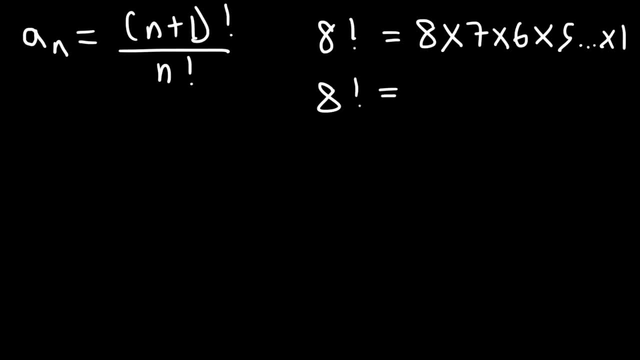 That's a factorial. Now you can also write a factorial as 8 times 7 factorial, Because 7 factorial is basically .7 times 6 times 5 times 4.. all the way to 1.. 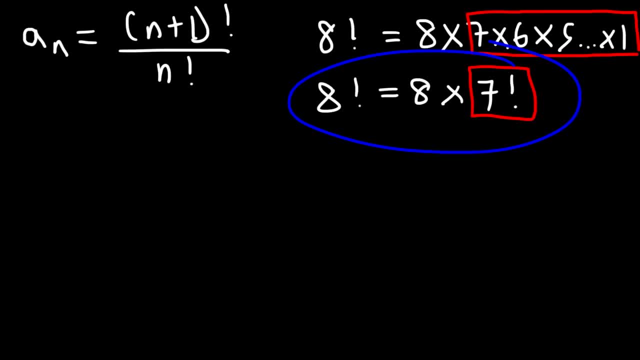 Now, this is the way in which we want to simplify a situation like this. So how can we change n plus 1 factorial? So notice, when we had 8. we started with the same number, 8.. 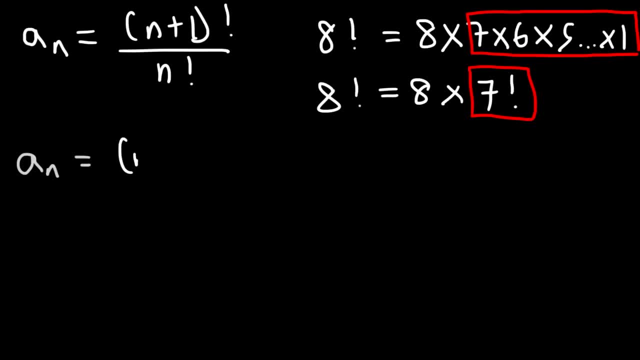 So here we have n plus 1.. We're going to start with n plus 1. Now to go from 8 to 7.. all we need to do is subtract it by 1. So to get the next one. 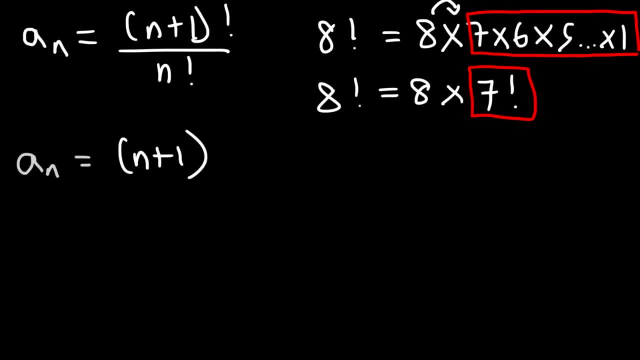 we just have to subtract n plus 1.. by 1.. n plus 1 minus 1 is n And we're going to write it like this. So this is going to be n factorial And the reason why we want to stop there. 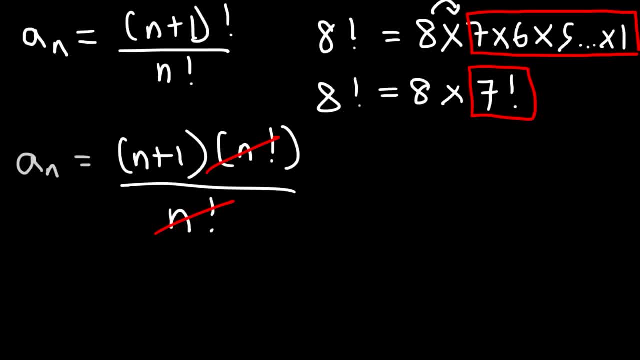 is because we can cancel these two, So we no longer have a factorial expression. So therefore, the limit as n approaches infinity for the original expression is equivalent to the limit as n approaches infinity. 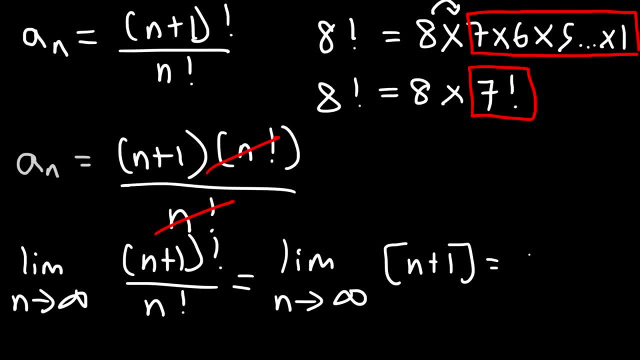 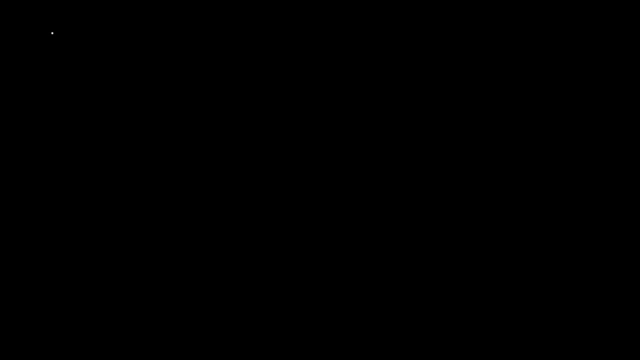 for n plus 1. And so infinity plus 1. is equal to infinity. So because the limit doesn't equal a specific constant, it equals infinity. the sequence diverges. Now let's try a similar problem. 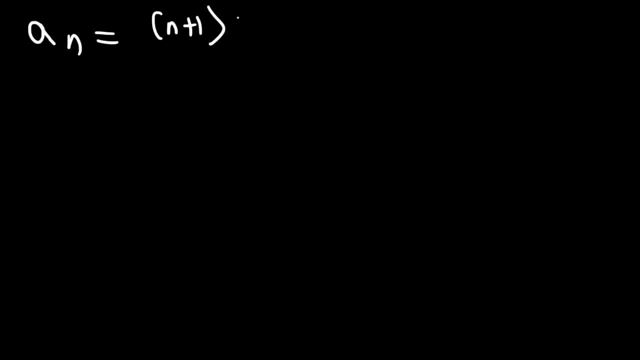 So this time it's going to be n plus 1 factorial divided by n plus 2 factorial. So feel free to pause the video and try it. So let's determine the limit as n approaches infinity. 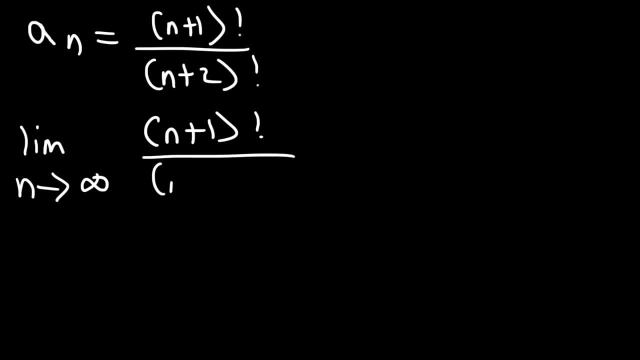 for this expression. Now, which one is larger: n plus 1 or n plus 2? n plus 2 is larger, so we're going to break that into two smaller parts. So let's start by rewriting the limit expression. 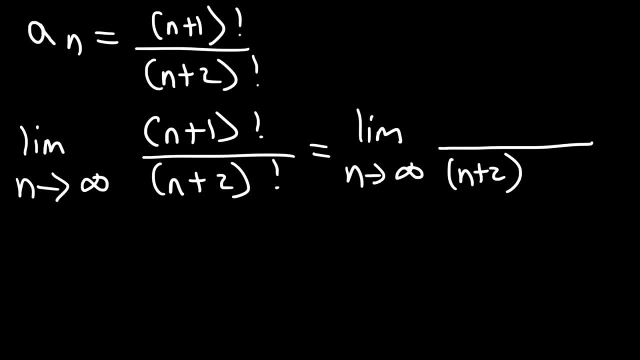 So we're going to have n plus 2.. and then if we subtract n plus 2 by 1.. minus 1 is 1.. So the next one is going to be n plus 1 factorial. 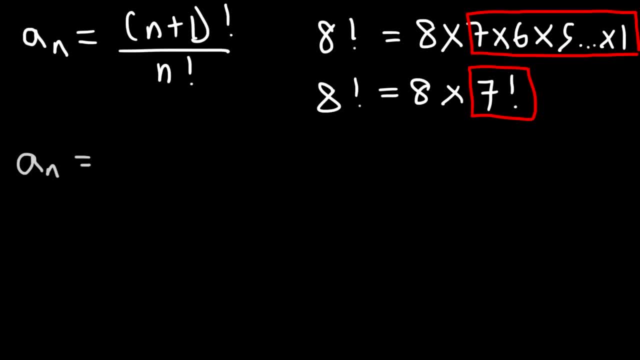 So how can we change n plus 1 factorial? So notice, when we had 8, we started with the same number, 8.. So here we have n plus 1.. We're going to start with n plus 1.. Now to go from 8 to 7, all we need to do is subtract it by 1.. 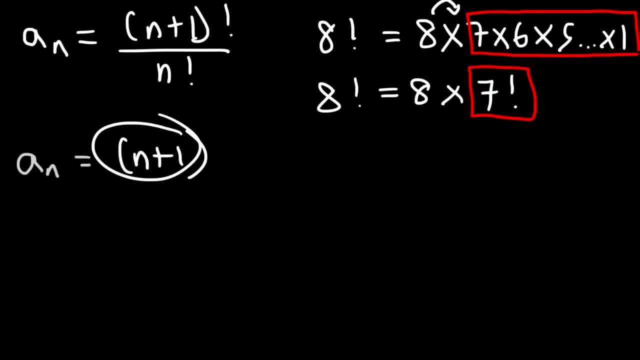 So to get the next one, we just got to subtract n plus 1 by 1.. n plus 1 minus 1 is n, And we're going to write it like this. So this is going to be n factorial, And the reason why we want to stop there is because we can cancel these two. 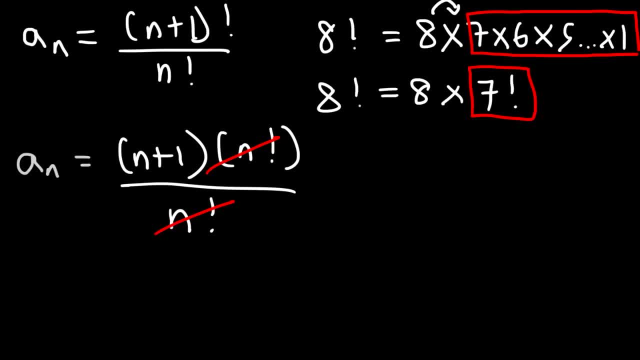 So we no longer have a factorial expression. So therefore the limit as n approaches infinity for the original expression is equivalent to the limit as n approaches infinity for n plus 1.. And so infinity plus 1 is simply infinity. So because the limit doesn't equal a specific constant, 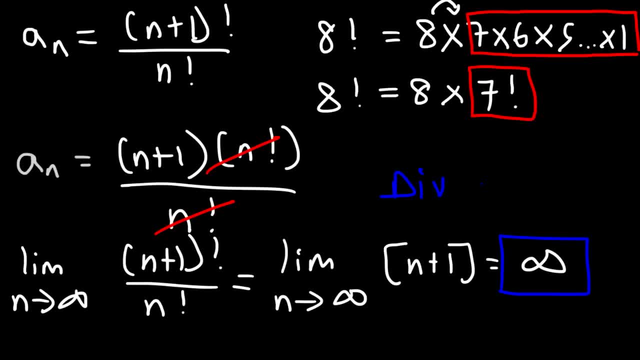 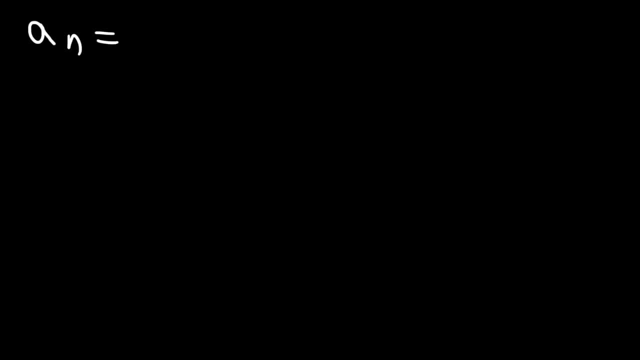 it equals infinity. the sequence diverges. Now let's try a similar problem. So this time it's going to be n plus 1 factorial divided by n plus 2 factorial. So feel free to pause the video and try it. 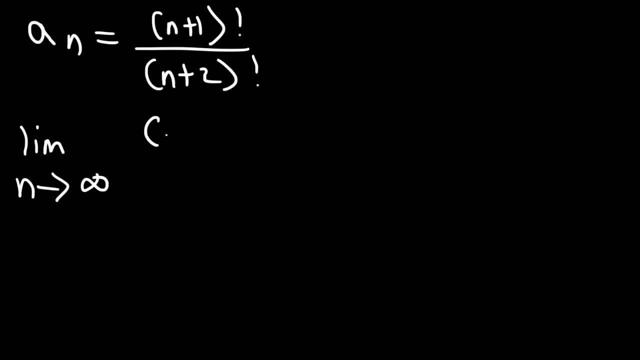 So let's determine the limit as n approaches infinity for this expression. Now, which one is larger: n plus 1 or n plus 2? n plus 2 is larger, so we're going to break that into two smaller parts. So let's start by rewriting the limit expression. 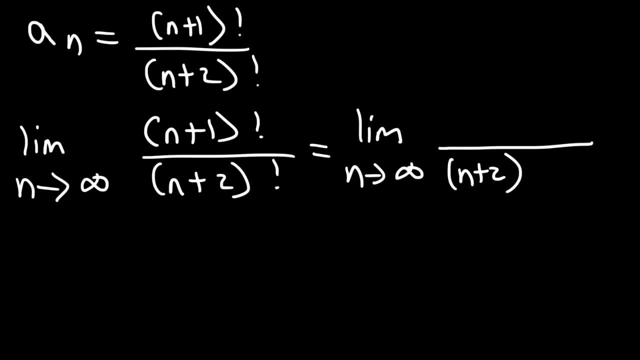 So we're going to have n plus 2, and then if we subtract n plus 2 by 1,, 2 minus 1 is 1.. So the next one is going to be n plus 1 factorial. So you want to do it in such a way that 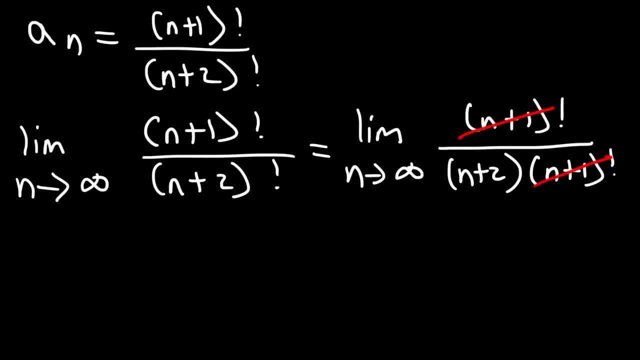 you could cancel out all the factorial expressions. So now we're left over with this: The limit as n approaches infinity for 1 over n plus 2.. And so if we multiply the top and the bottom by 1 over n, 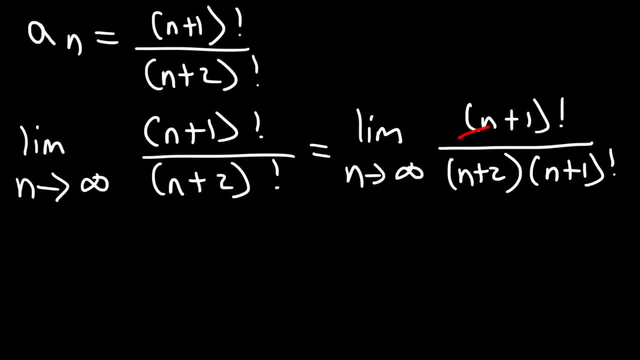 So you want to do it in such a way that you could cancel out all the factorial expressions. So now we're left over with this: The limit as n approaches infinity for 1 over n plus 2.. And so if we multiply, 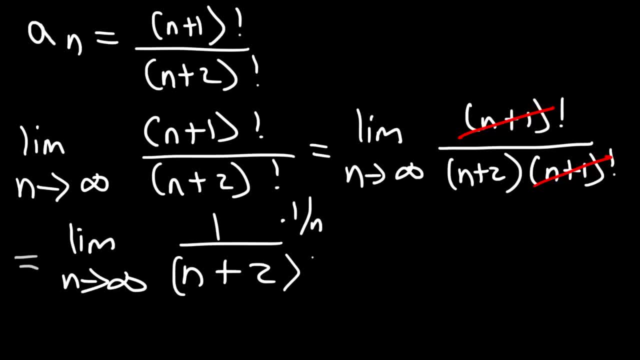 the top and the bottom by 1 over n. we're going to get this. So it's 1 over n and then n times 1 over n. that's just going to be 1.. 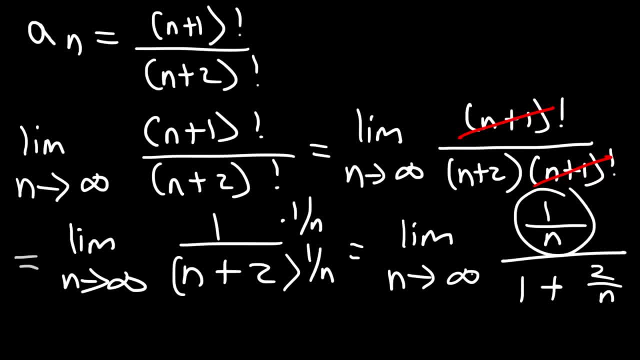 plus 2 over n. So anytime you have a constant over n, as n approaches infinity, it's going to be 0. So we're going to have 0 over 1 plus and then 2 over n. 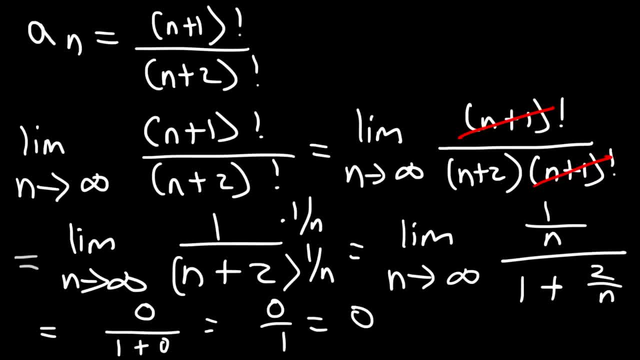 that's going to go to 0.. So this becomes 0 over 1, which is 0.. So the limit for this entire thing is 0,, which means that the sequence is going to converge. 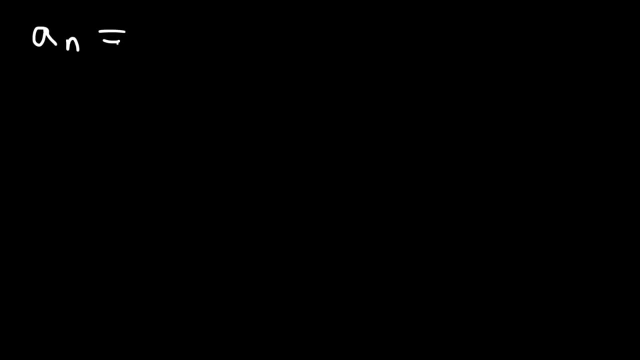 So here's another problem for you. Let's say that a sub n is equal to 4n divided by the square root of n squared plus 5.. So go ahead and see if this sequence 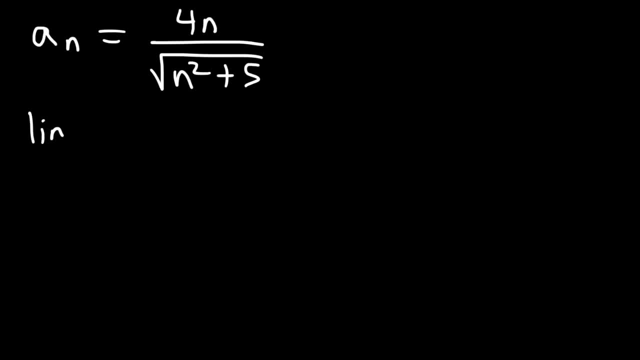 is going to converge. So how can we determine the limit, as n approaches infinity, of 4n divided by the square root of n squared plus 5?? So, for this example, all we need to do 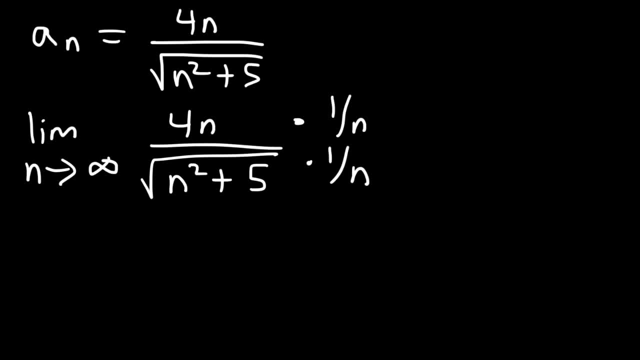 is: multiply the top and the bottom by 1 over n. Now what you need to know is that .1 over n is the same as the square root of 1 over n squared. So what we're going to do is: 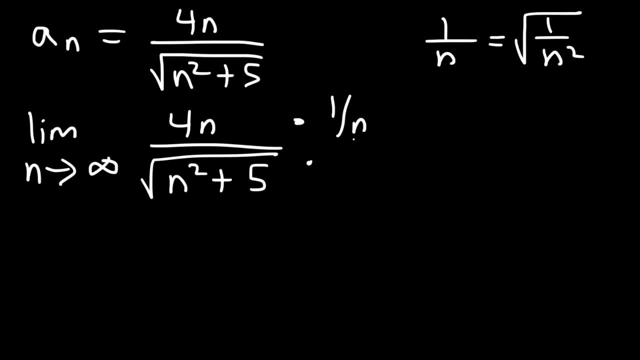 replace 1 over n on the bottom with the square root of 1 over n squared. So now we can multiply by the contents of the stuff inside the square roots. So 4n times 1 over n. 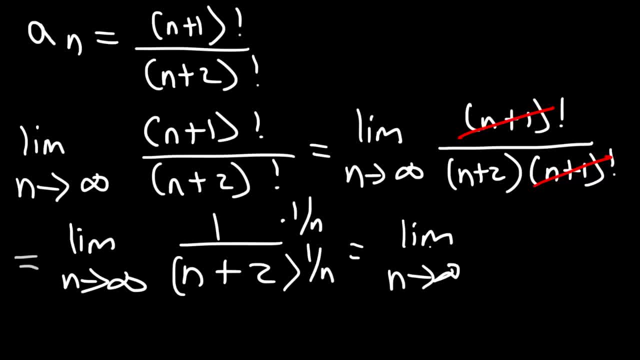 we're going to get this. So it's 1 over n and then n times 1 over n. that's just going to be 1, plus 2 over n. So anytime you have a constant over n as n approaches infinity. 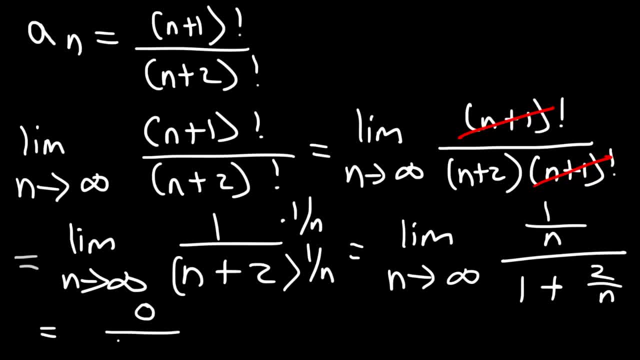 it's going to be 0. So we're going to have 0 over 1, plus, and then 2 over n. that's going to go to 0. So this becomes 0 over 1, which is 0.. 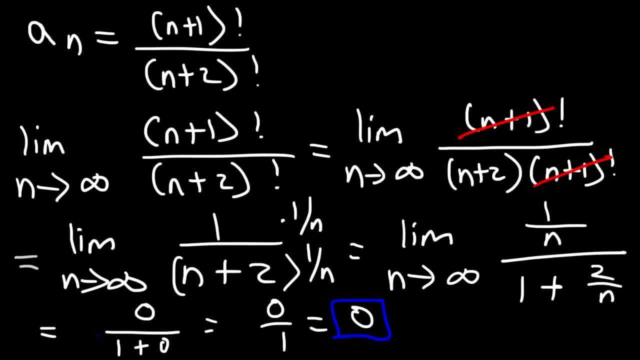 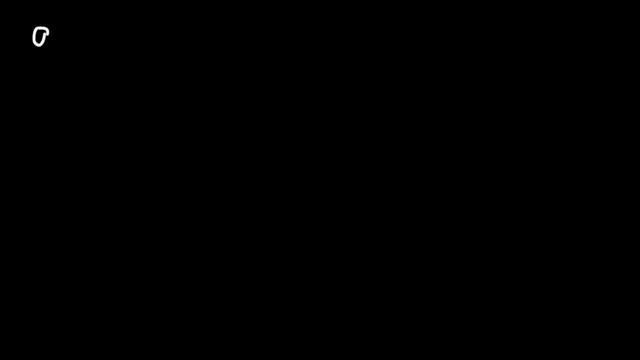 So the limit for this entire thing is equal to 0, which means that the sequence is going to converge. So here's another problem for you. Let's say that a sub n is equal to 4n divided by the square root of n squared plus 5.. 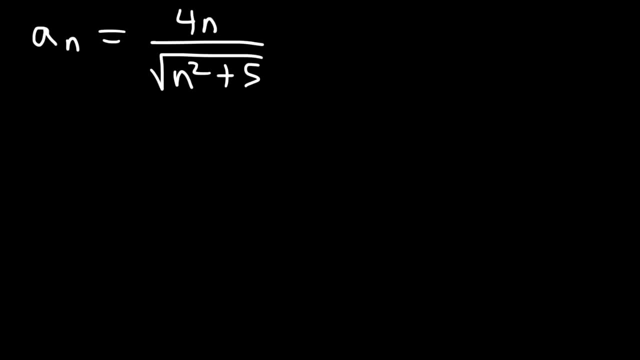 So go ahead and see if this sequence is going to converge. So how can we determine the limit, as n approaches infinity, of 4n divided by the square root of n squared plus 5?? So for this example, all we need to do is multiply the top and the bottom. 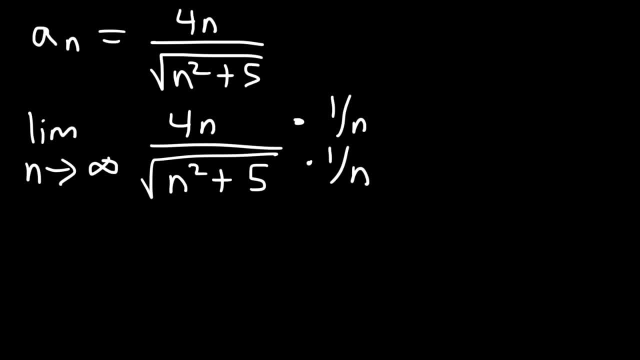 by 1 over n. Now what you need to know is that 1 over n is the same as the square root of 1 over n squared. So what we're going to do is replace 1 over n on the bottom with the square root. 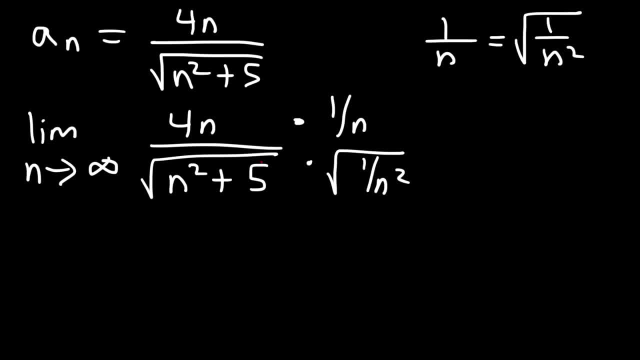 of 1 over n squared. So now we can multiply by the contents of the stuff inside the square roots. So 4n times 1 over n, that's just going to be 4.. And then n squared times n squared, that's 1.. 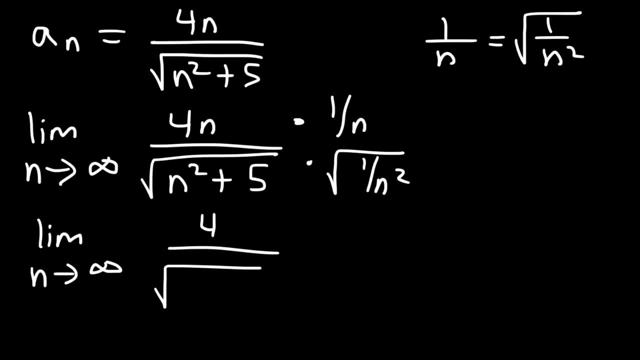 that's just going to be 4.. And then n squared times 1 over n squared, that's 1.. And then we're going to have .5 over n squared. So at this point I'm going to rewrite the expression like this: 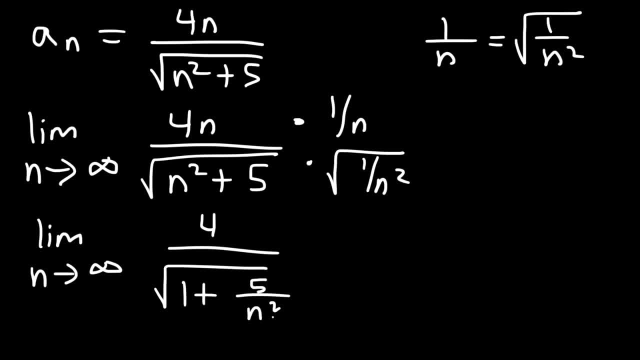 And then we're going to have 5 over n squared. So at this point I'm going to rewrite the expression like this: So it's 4 divided by the square root of 1 plus 5 times 1 over n, times another 1 over n. 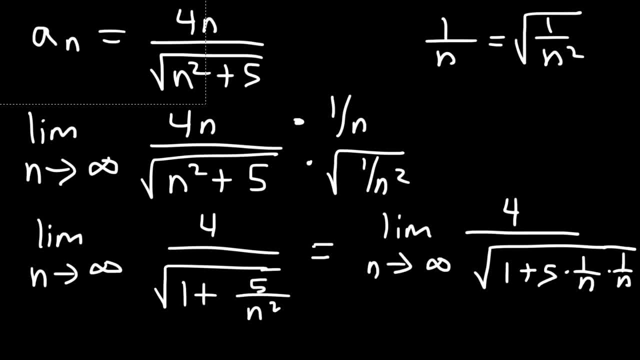 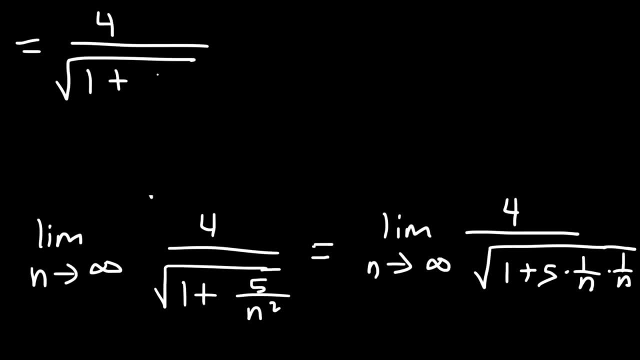 So that's the same as 5 over n squared. So now we can apply the limit expression. We know that the limit as n approaches infinity for 1 over n is 0. So this becomes 4 divided by the square root of 1 plus. 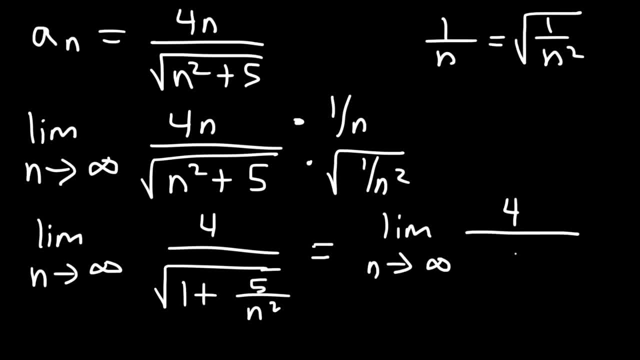 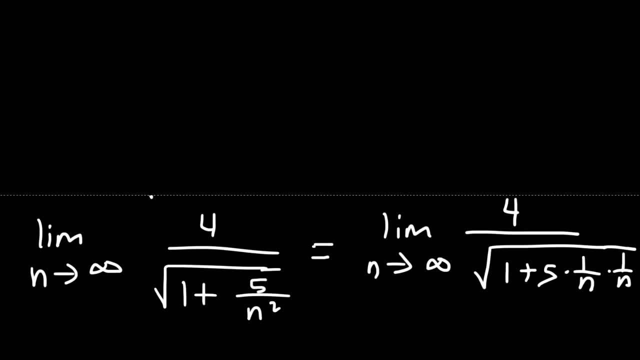 So it's .4 divided by the square root of 1. plus 5.. times 1 over n, times another 1 over n, So that's the same as 5 over n squared. So now, 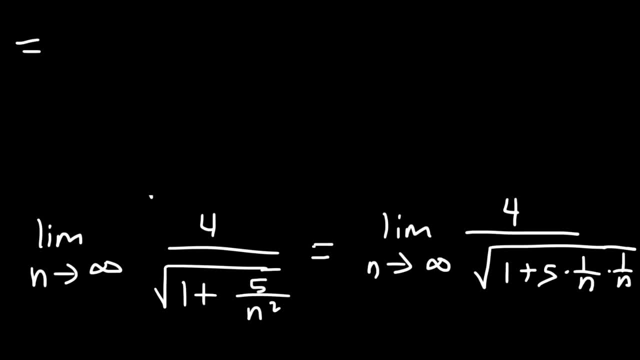 we can apply the limit expression. We know that the limit as n approaches infinity for 1 over n is 0. So this becomes 4. divided by the square root of 1 plus 5 times 0.. 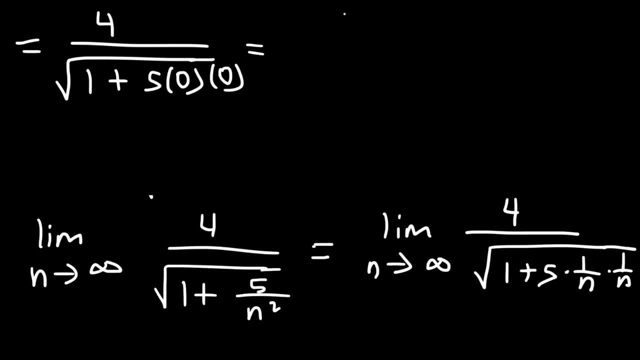 And then the other 1 over n is 0 as well. So we're going to have 1 plus 0.. which is 1.. And the square root of 1 is 1.. So the whole thing is equal to 4.. 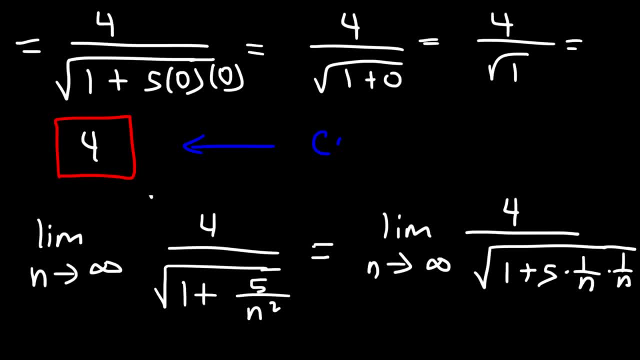 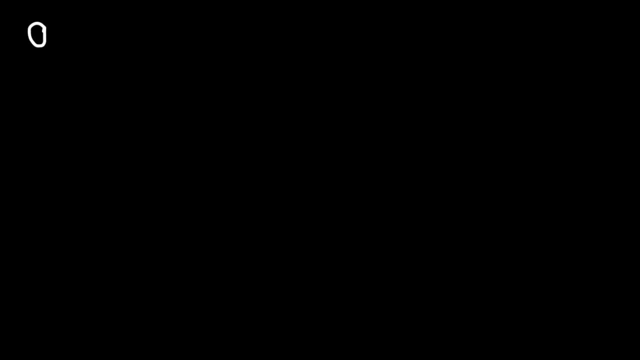 Therefore, the sequence converges, And so that's all we need to do for this problem. Now let's try one more problem. So let's determine if the sequence is going to converge. if we have. 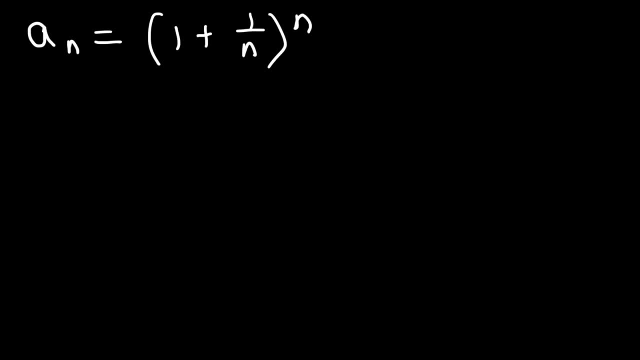 .1 plus 1 over n raised to the n. So go ahead and try that. So how can we determine the limit as n approaches infinity for that expression? Well, to do so, we need to set this entire limit. 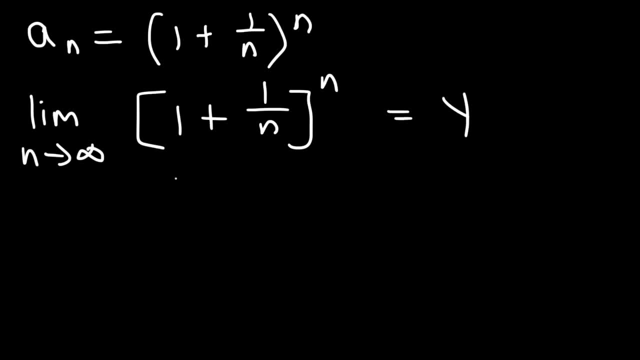 equal to a variable. Let's call it y, And then we're going to take the natural log of both sides, So I'm going to put this back on the left, So I'm going to have the natural log of y. 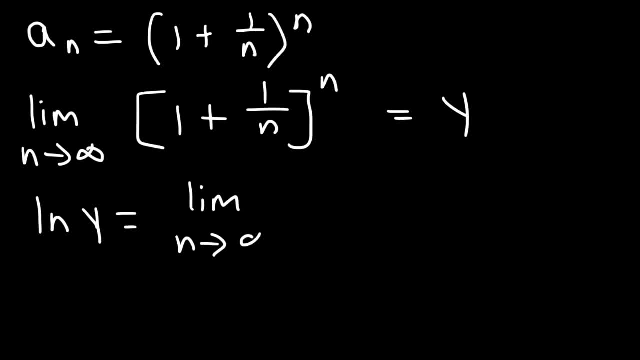 is equal to the limit, as n approaches infinity, of the natural log of 1 plus 1 over n raised to the n. Now, the reason why I need to do this is so that I can take this: 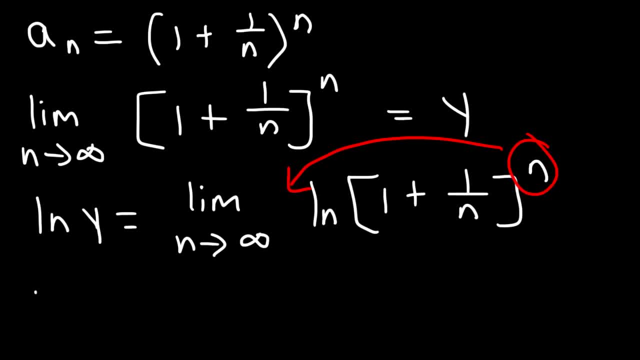 variable and move it to the front. So now what I have is l and y is equal to the limit as n approaches infinity n times the natural log of 1 plus 1 over n. 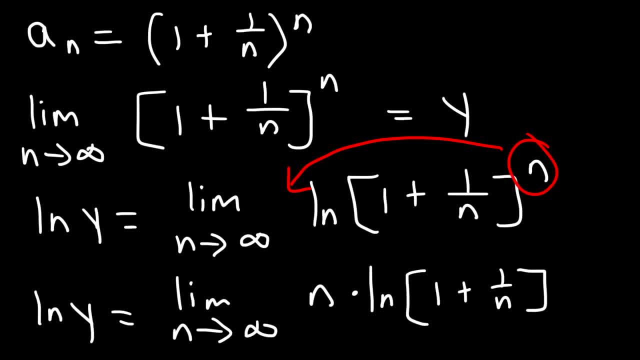 Now I need to use L'Hopital's Rule, but I need to convert it into a form in which I could use L'Hopital's Rule, So I have to change it from multiplication to division. 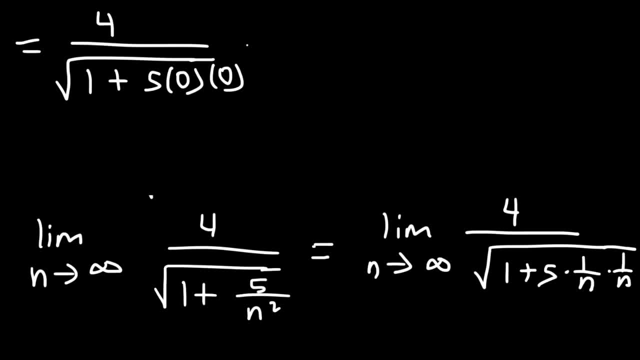 5 times 0.. And then the other 1 over n is 0 as well. So 5 times 0 is 0. So we're going to have 1 plus 0, which is 1.. And the square root of 1 is 1.. 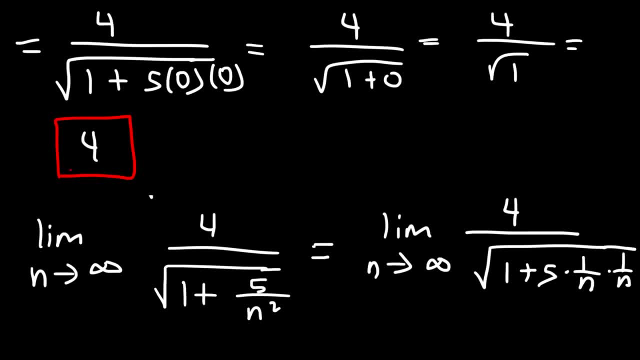 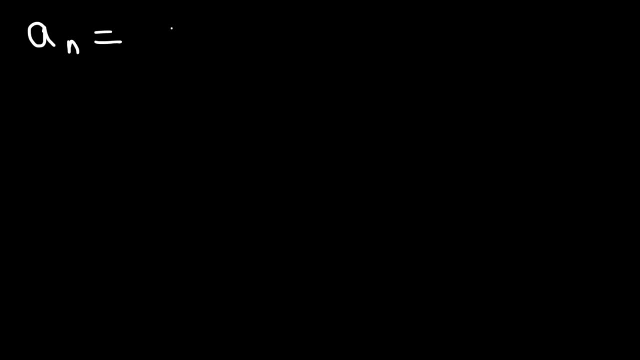 So the whole thing is equal to 4.. Therefore, the sequence converges, And so that's all we need to do for this problem. Now let's try one more problem. So let's determine if the sequence is going to converge. if we have 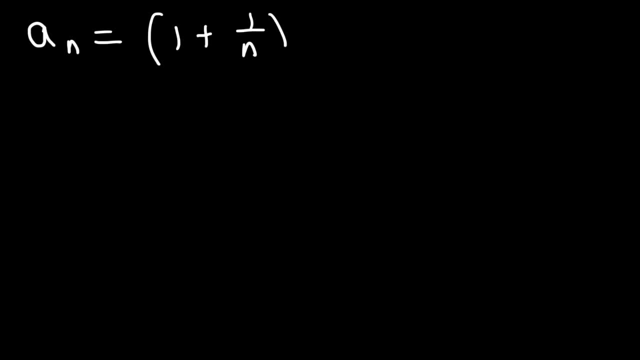 1 plus 1 over n raised to the n. So go ahead and try that. So how can we determine the limit as n approaches infinity for that expression? Well, to do so, we need to set this entire limit equal to a variable. 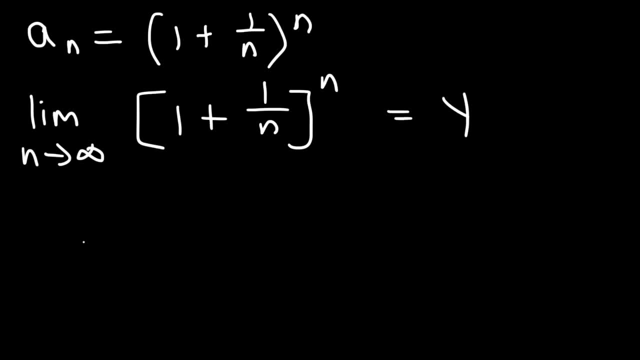 Let's call it y, And then we're going to take the natural log of both sides. So I'm going to put this back on the left. So I'm going to have: the natural log of y is equal to the limit as n approaches infinity. 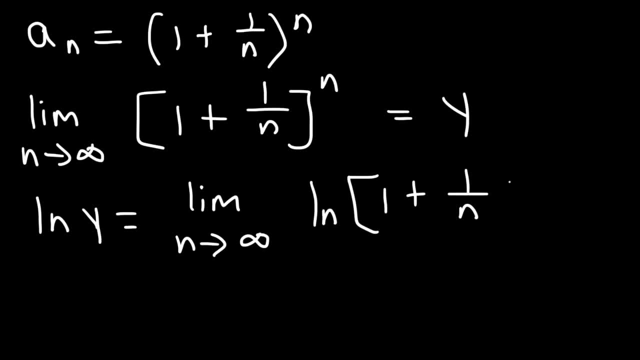 of the natural log of 1 plus 1 over n raised to the n. So what I'm going to do is so that I can take this variable and move it to the front. So now what I have is l and y is equal to the limit. 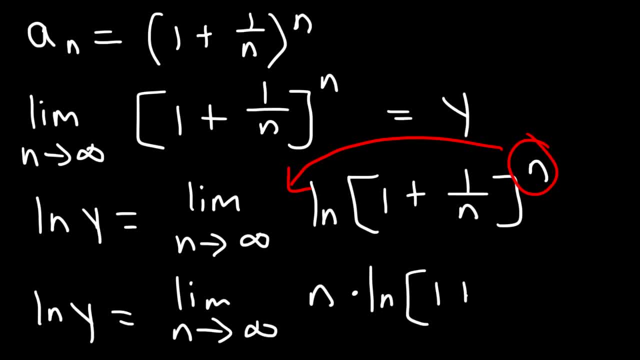 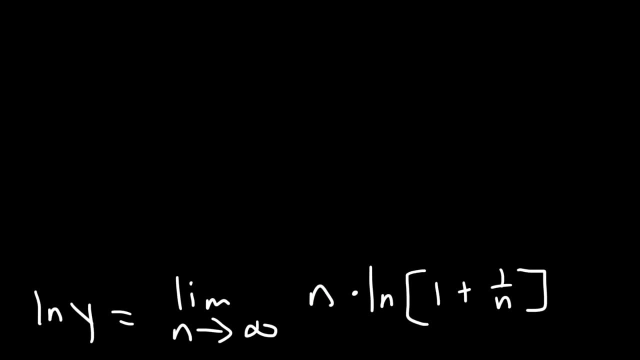 as n approaches infinity, n times the natural log of 1 plus 1 over n. Now I need to use L'Hopital's Rule, but I need to convert it into a form in which I could use L'Hopital's Rule, So I have to change it from multiplication. 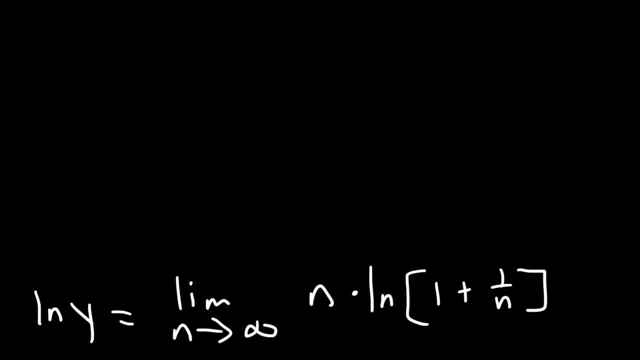 to multiplication. So keep in mind: n is the same as 1 divided by 1 over n. So now we have that l and y is equal to this limit of ln, 1 plus 1 over n divided by 1 over n. So now let's find: 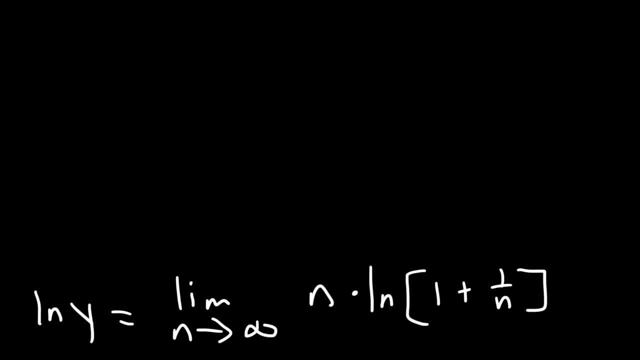 So keep in mind n is the same as .1 divided by 1 over n. So now we have that l and y is equal to this limit of ln, .1 plus 1 over n. 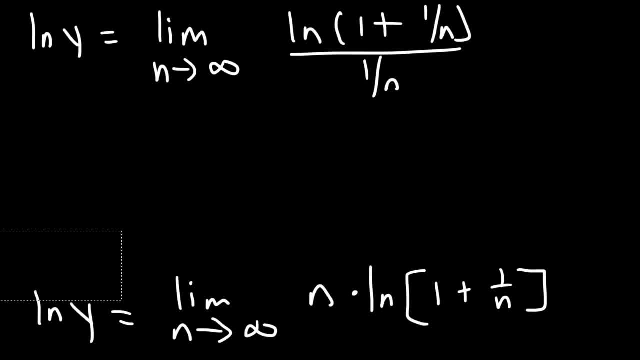 divided by 1 over n. So now let's find the derivative of the top and the bottom of the fraction. So we're going to have l, and y is equal to this. Now we know that the derivative of 1 over n. 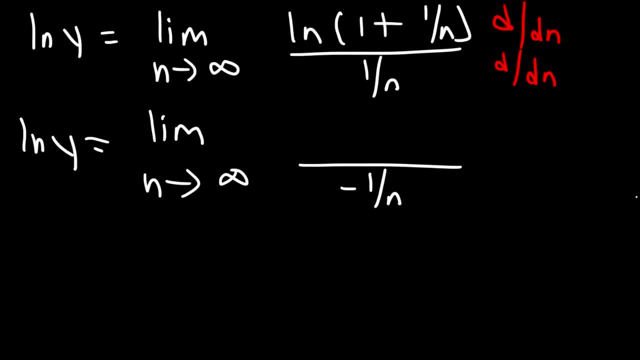 is negative, 1 over n squared. And to differentiate a natural log function, let's say l and u, it's going to be u prime divided by u. So u is 1 plus 1 over n, The derivative of 1 plus 1 over n. 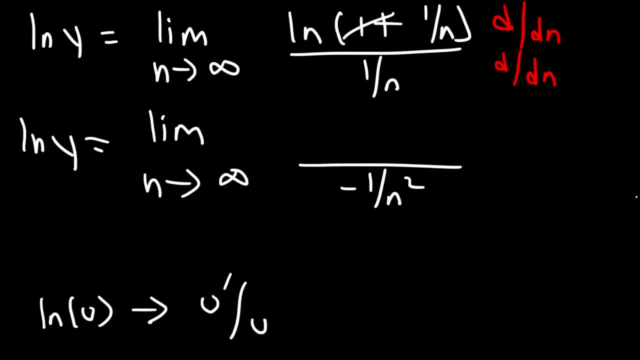 the 1. basically turns into 0. And then, differentiating 1 over n, that's going to be negative, 1 over n squared- And then it's going to be divided by u. So u is just the stuff. 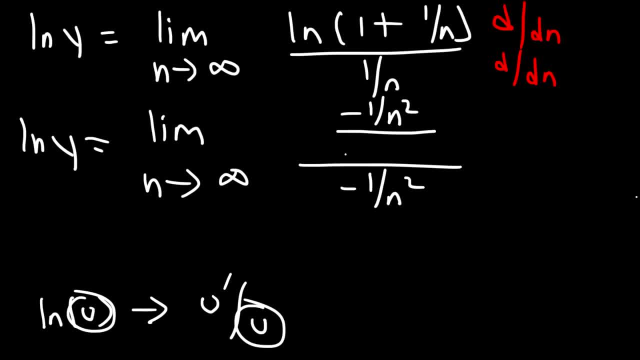 that's on the inside of the ln function, And so that's going to be 1 plus 1 over n. Now you can put this over 1. if you want. but this is the big fraction, so to speak. 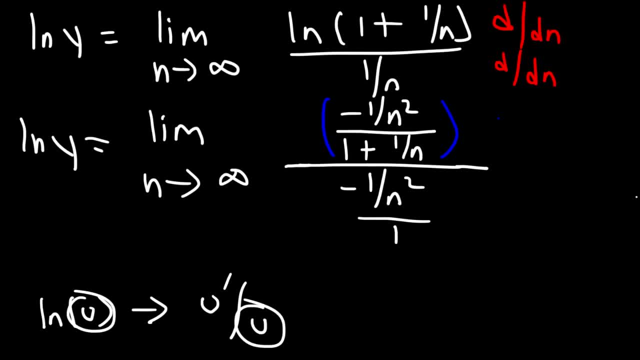 Now we're going to multiply this fraction by negative n squared And this fraction also by negative n squared. So negative 1 over n squared times negative n squared. they will cancel, Leaving behind just positive 1.. 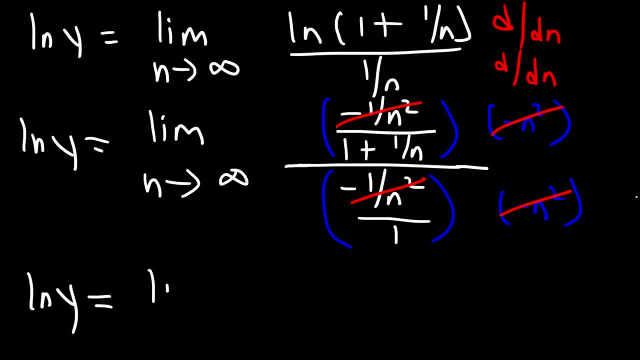 And so now we have the natural log of y is equal to the limit as n approaches infinity, And so we have .1 over .1, plus 1 over n, And this part, this whole thing, becomes 1, so 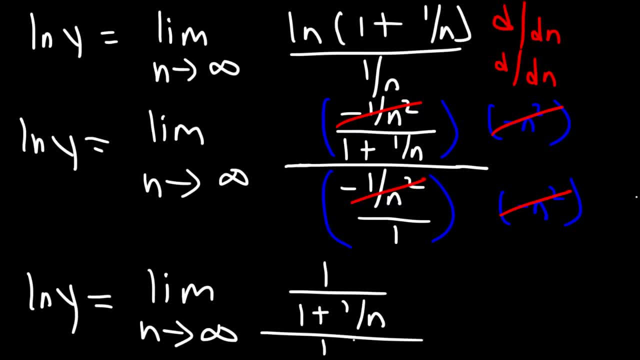 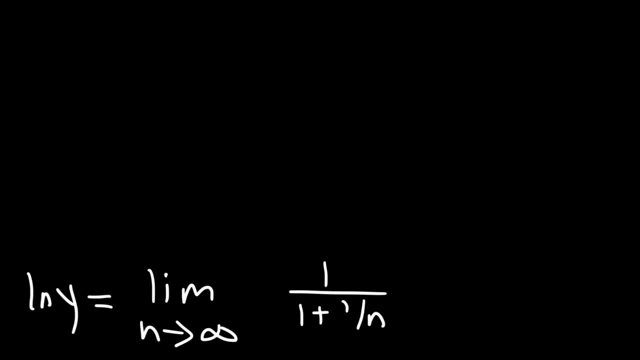 we don't need to write that. If you want to write it like this, you could, but there's no point. So now we can apply the limit expression to 1 over n, Which is 0. So we're going to have ln. y is equal to. 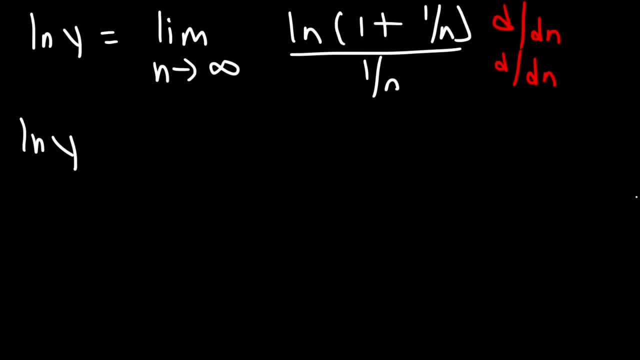 the top and the bottom of the fraction. So we're going to have l, and y is equal to this. Now we know that the derivative of 1 over n is negative- 1 over n squared- And to differentiate a natural log function, let's say l and u. 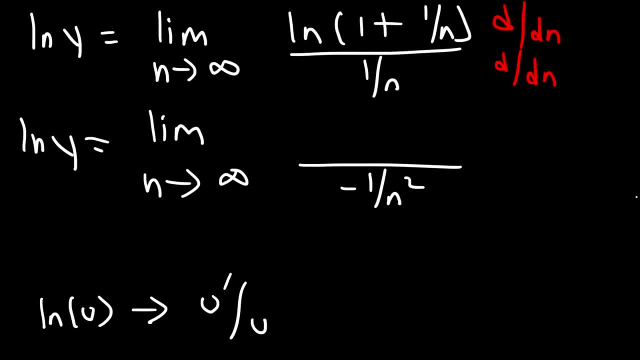 it's going to be u prime divided by u. So u is 1 plus 1 over n, The derivative of 1 plus 1 over n. that's going to be negative 1 over n squared. And then it's going to be divided by u. 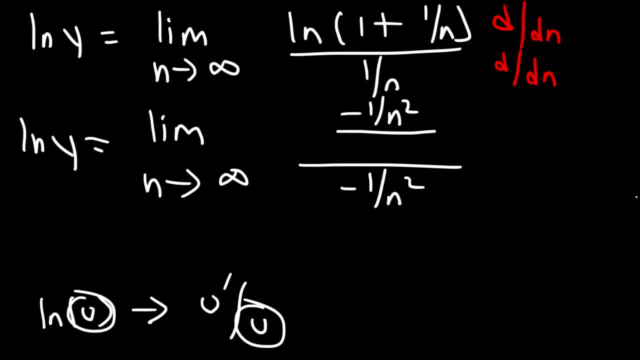 so u is just the stuff that's on the inside of the ln function, and so that's going to be 1 plus 1 over n. Now you can put this over 1 if you want, but this is the big fraction, so to speak. 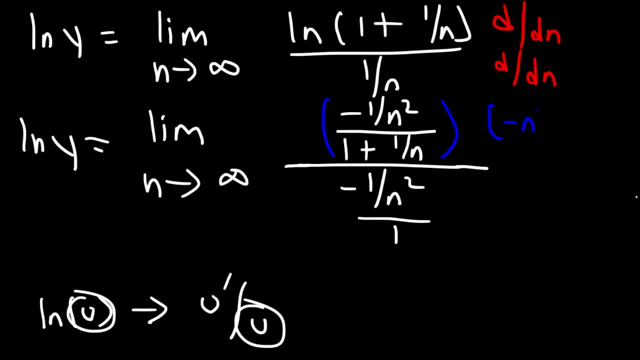 Now we're going to multiply this fraction by negative n squared and this fraction also by negative n squared, So negative 1 over n squared plus negative n squared. they will cancel, leaving behind just positive 1.. And so now we have the natural log of y. 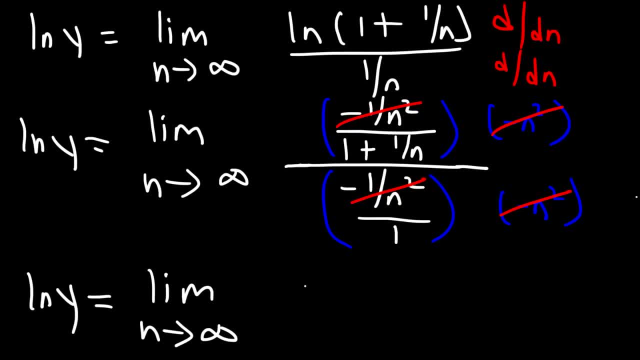 is equal to the limit as n approaches infinity, and so we have 1 over 1 plus 1 over n, And this part, this whole thing, becomes one. so we don't need to write that. If you want to write it like this, you could. 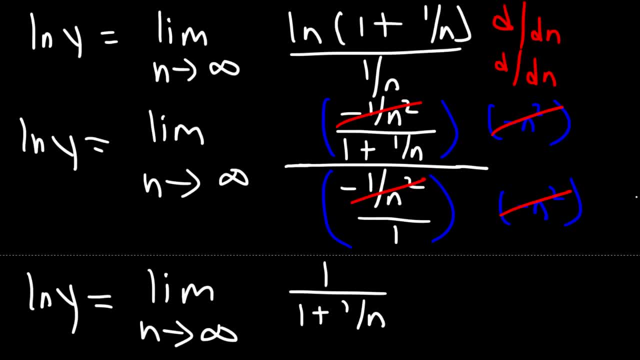 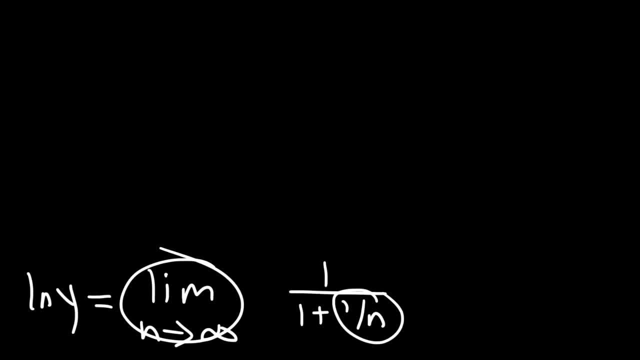 but there's no point. So now we can apply the limit expression to 1 over n, which is 0. So we're going to have: ln. y is equal to 1 over 1 plus 0. And so 1 plus 0 is just 1. 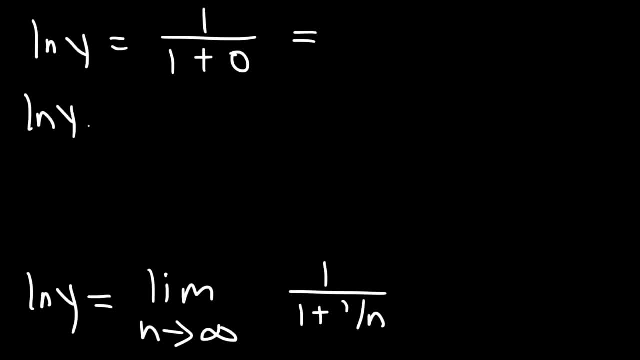 1 divided by 1 is 1, so ln y is equal to 1.. Now the base of the natural log function is e, So we can say e to the first power is equal to y. So therefore the limit as n approaches infinity.